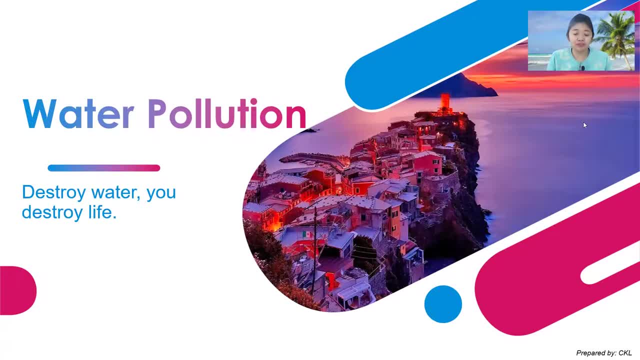 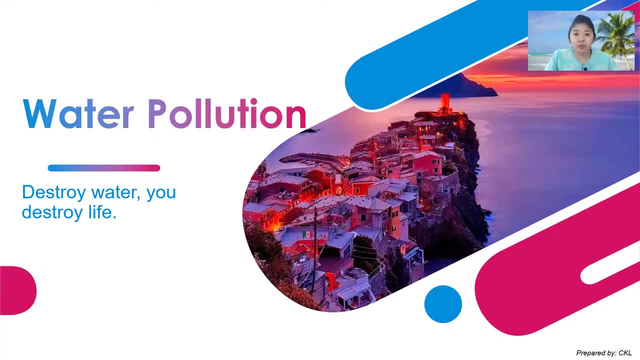 everyone of you will have and you know what is water pollution, such as, example, you will say, throw the rubbish into the river. So, and then those who stay in Selangor, currently, those who stay in Selangor, who, those who in Klang KL, you are quite often facing the 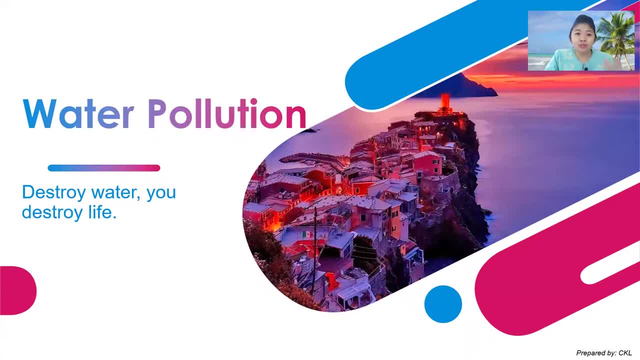 water pollutions impact, So those impacts will cause you have no water supply. Okay, so you will know how important the water is. it All right. So today's our chapters will be on water pollutions. So when we say about water pollutions, why this is? 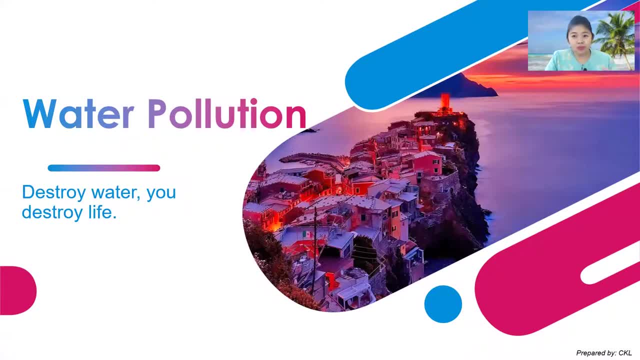 Because when we destroy our water, that means you are destroy your own life. Can we survive without any water? Okay, so can we survive without any water? Definitely not. Every day is when you are wake up, you need water. When you, before you sleep, you need to drink water. Even while you are eating. 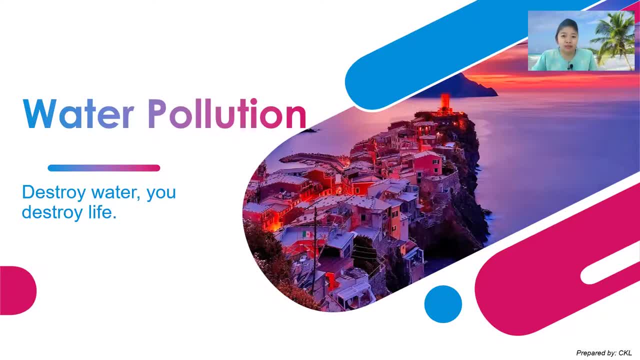 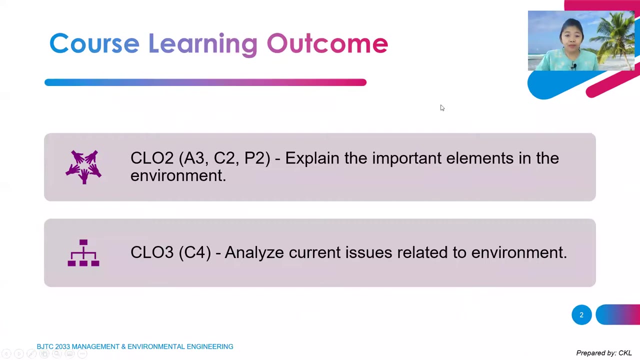 you need water And talking like this, also I need a lot of water. So when your water's been gone. so it means if we are destroying water, that means we are destroy our own life. Okay, so right. So for these chapters, the course learning outcomes will be the CLO 2 and then also CLO 3,. 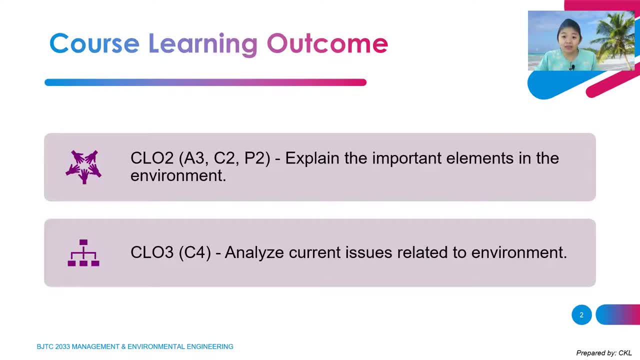 which is to help you explain. You will at least need to explain the important element in the environments. So do the training and so on. and you have to do the course on that, So the course on what the outcomes are, and so on. and then also the CLO 3, and then also the CLO 4, which is to help you. 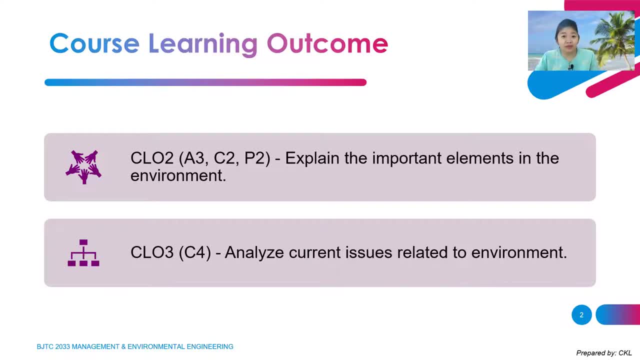 explain. you will at least need to explain the important element in the environment. That means what is the important elements in the environments? in these chapters It's the waters, What is important. Then some things that you need to learn how to explain it okay. 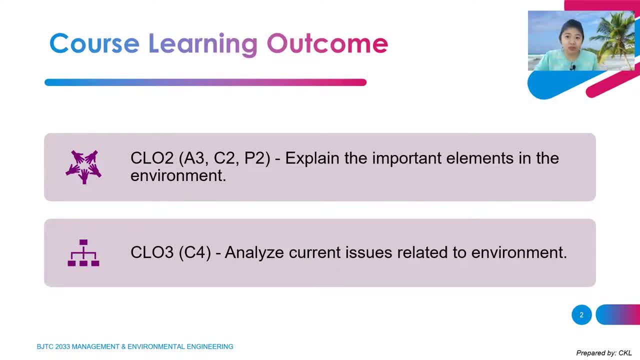 Because you didn't have finals. Usually the finals questions were based on this, okay, So I will ask you what is the important? You will need to identify this, okay. So, secondly, is you need to analyze the current issues that relate to the environment? 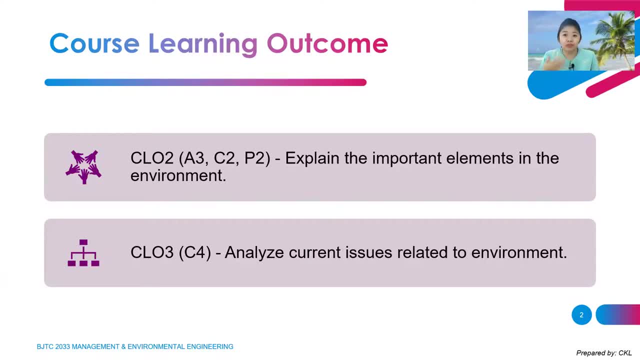 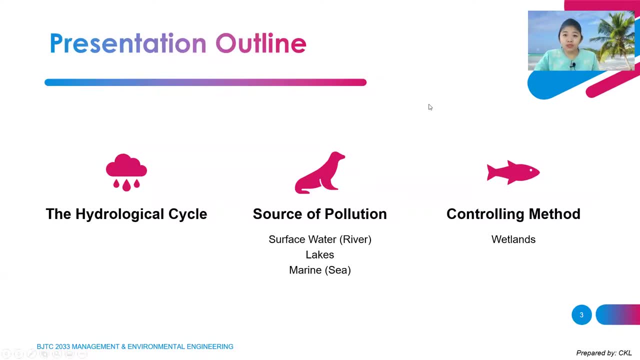 So what is the current issue that relates with the waters or water pollution? So you need to know what is the current issues. okay, Right, So today's presentation outlines. we will have three main parts that we need to learn, okay. 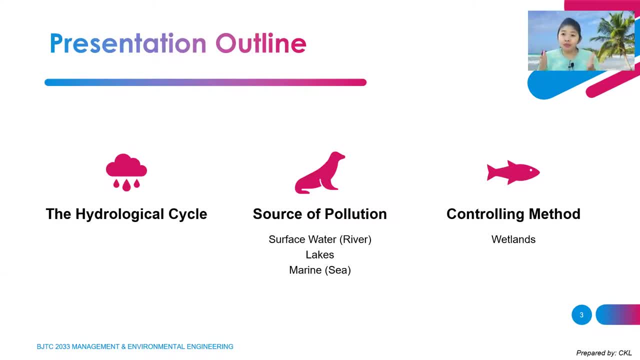 First, I need to tell you, before the water you can use, so before the pollution happens, what it means by a water. What is a water? okay, Some things that you need to understand first. So that is the hydrological cycles. 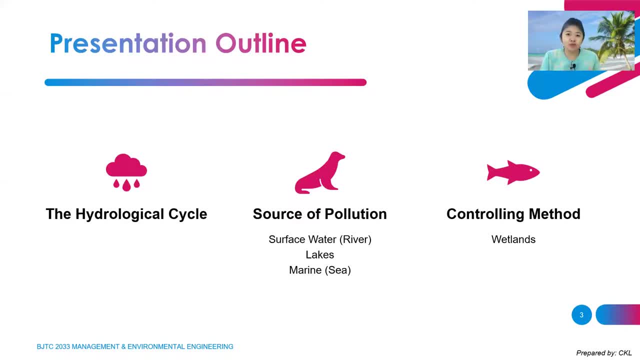 You need to understand the cycle, the whole cycle, And I'm sure all of you have the basic idea of the cycles Because you've been learning through your science class since your primary to your secondaries, until now. okay, So this is some things that you've been learning. 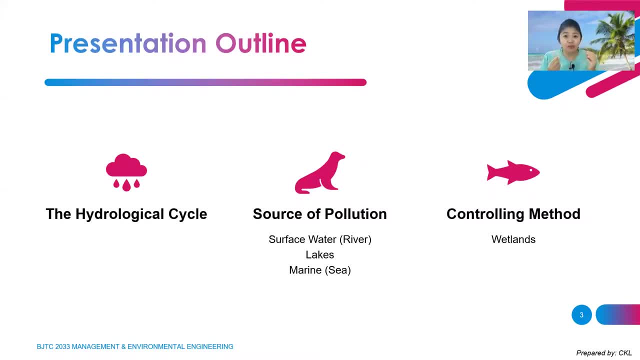 But then I just want to recap you, And then there are some small parts that, while you are learning, previously maybe you didn't notice that, okay, So second. Second is the source of pollutions. When we say about the water pollutions, we not only have one types of water, okay, 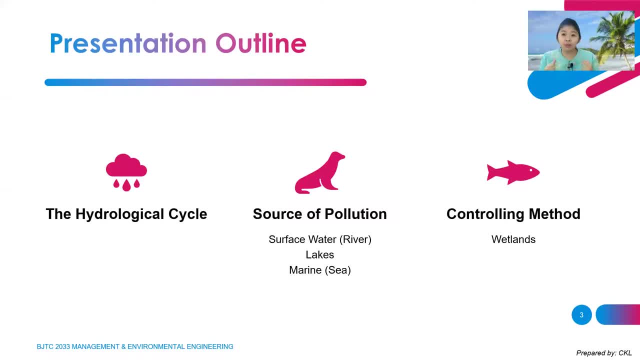 Generally, every one of us think: okay, our waters come from our tape water. So when you open your tape, then that is the waters, But you have your other things. Where is this water coming from? okay, When you say it's coming from the station, so from where the stations get the waters? 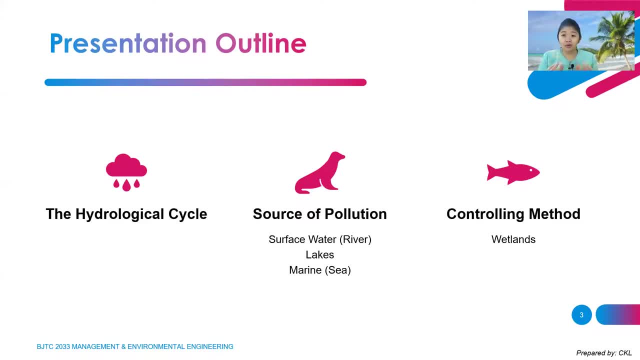 When you say it's coming from the station. so from where the stations get the waters You said about, like the cases in Selangor, the water stations been destroyed, So from where the water is coming from. So we have to know from the early starting. okay, 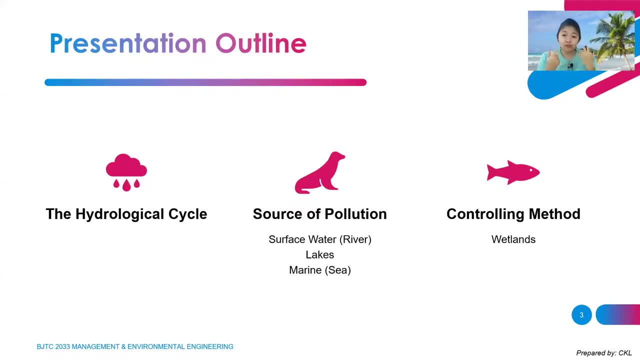 The starting parts of the waters. okay, So the source of the pollutions or the source of the water, we actually have three types. So we have three types of water that we take the waters, okay, First is actually from our river. 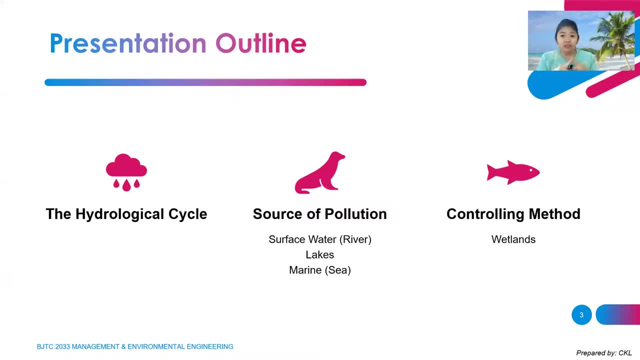 So we have the river water. Second is our lake. Second is our lake, So we have lake water. As an example for northern regions at least, we have Timatasso. That is one of our place, the lake that we store our water. 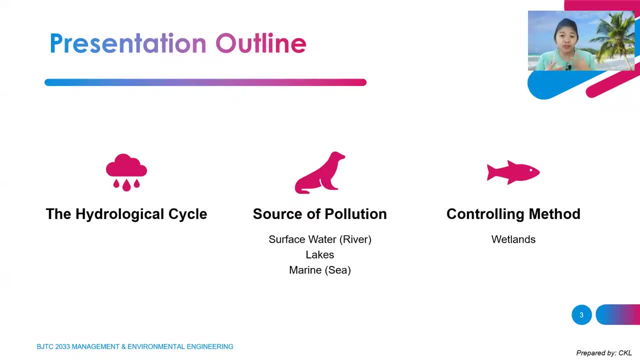 For Kedah we have Tasik, Pedu Pedu Lake, And then for Tengganu we have Kenyan Lake. So all those, that very famous lake is actually our source. So what happens if here the source of the water is polluted? 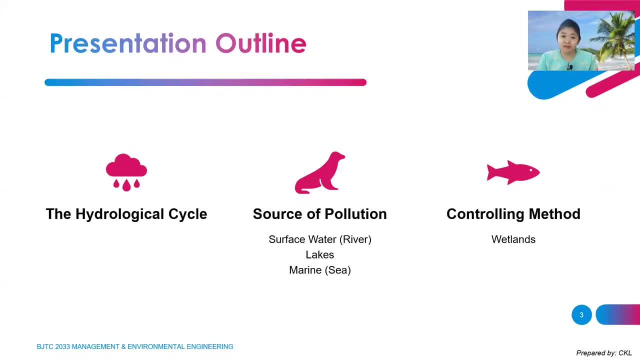 So what happens to us? So the last one is the seawater, which is marine Seawater in Malaysia. we didn't implement it or we didn't use it, but it happens to our closer country, Singapore. Singapore is an island. 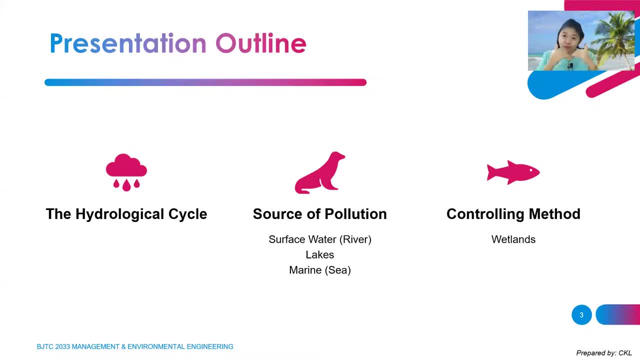 So even when the rain drops, the waters cannot store. So all the waters that They receive- your water is actually from Malaysia. We pump in the water for them, We send the waters for them. Beside that, they also have. They take the seawater and then they process and make it as a drinking water. 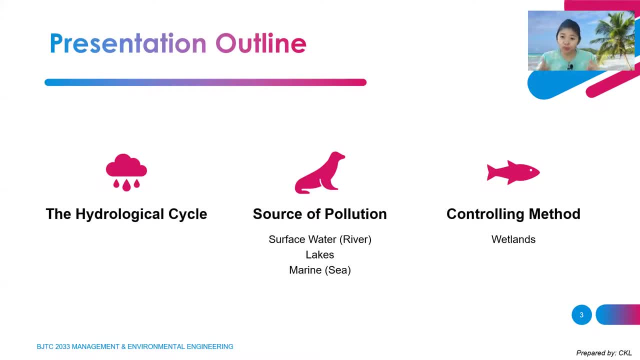 So the name of the water is called as the new water. You can try to search: It's called as a new water. And then, finally, how are we going to control the pollution? How are we going to help to avoid the pollution? 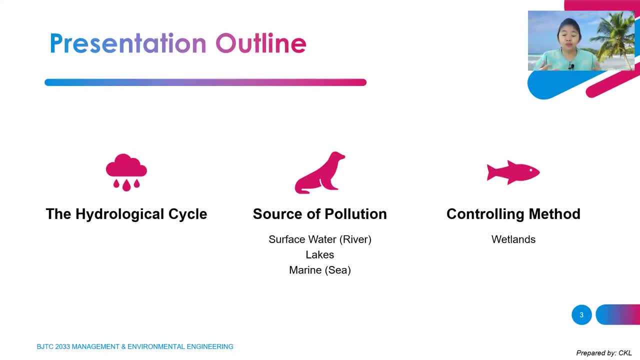 Sometimes you didn't thought that that is, The actions that you do is actually one of the pollutions method. It's one of the things that you pollute to our source, But then, so from these chapters you will understand how we've been polluted. 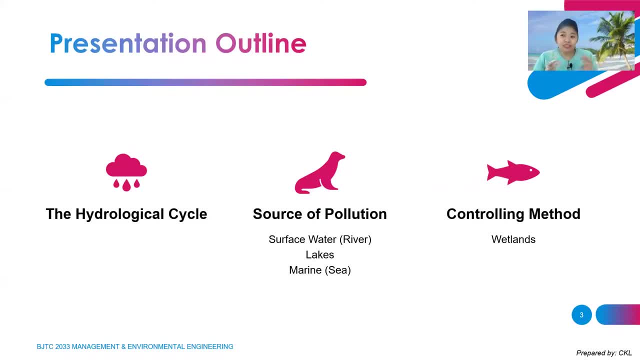 and then how we're going to control. It's actually Nature is something that's very unique. It can have the pollutions and then it actually have the energies or the abilities to self-recover. So it's just an example. When you are sick, sometimes you didn't want to take the medicine. 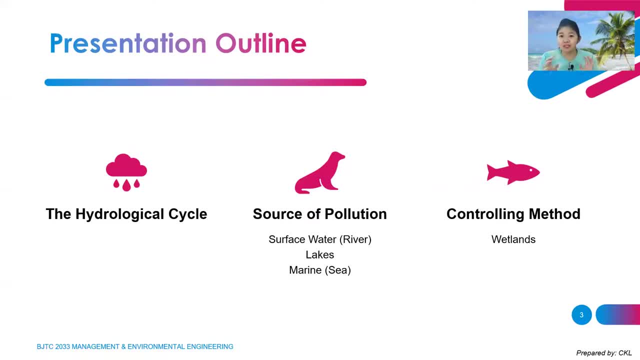 So you recover by yourself. So it's the same concept. So from this I will tell you, So one is polluted, how it recovers. But if in a big quantity, that means all of this cannot be Done, Okay. 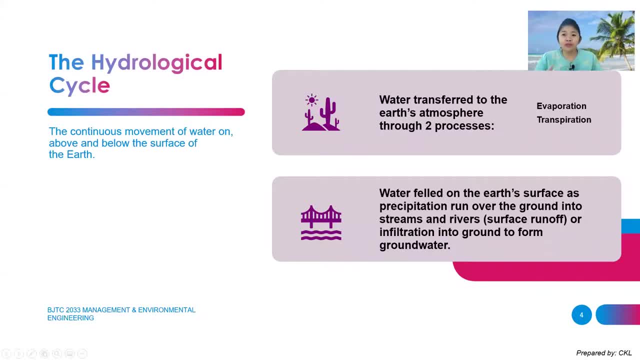 Right, So enters to the first, where we talk about hydrological cycles. So hydrological cycle is Kitaran hydrology. I'm sure it's quite familiar for you guys. So the definition is: Wait, let me get my pen, Okay. 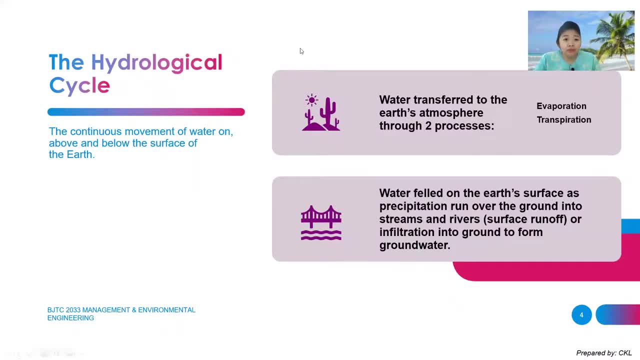 So you can see from here Where is my pen. Okay, All right. Okay, So we will see. from here, You can see. Okay, So the hydrology cycles mean the continuity, Okay, Continuous movement of water on above, on above and below the surface of the earth. 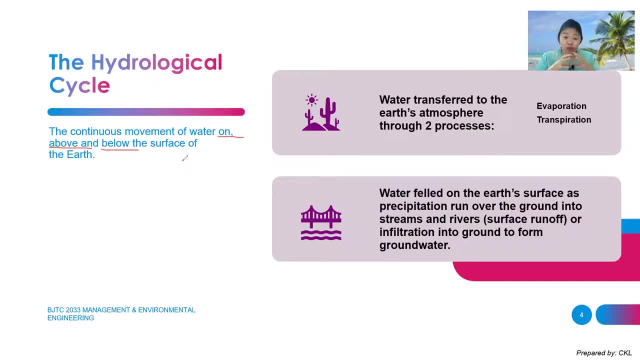 Okay, So this is our earth, The water that having on the surface, Okay, Above the surface, which is above of us, Such as example Now on the surface from my fingers, you can see. Okay, The water in the river is on the surface. 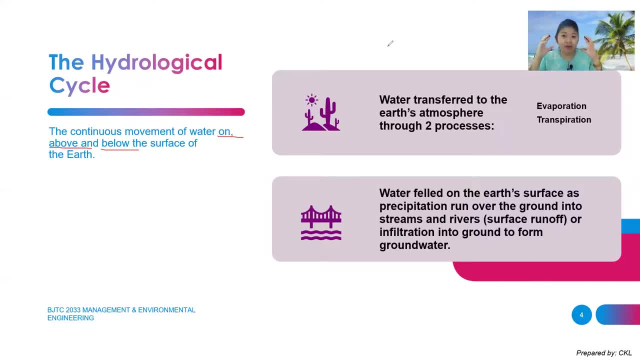 The water at the cloud is on the surface, Above the surface, Okay, Underground waters, Waters that you drinks in, the drinking water, Let's say your mineral water. This is below the surface, which is where we call it as the underground water. 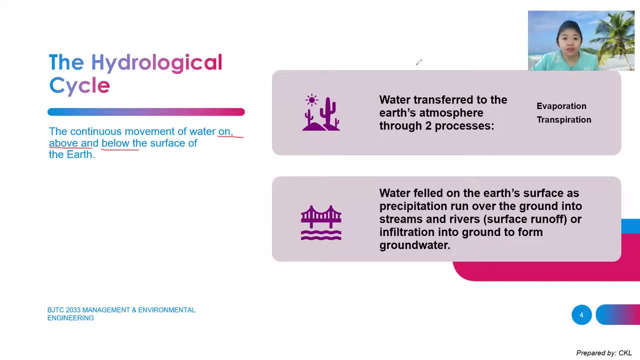 Okay. And then also, you see, The waters will be transferred to the earth atmosphere through the two process. One is evapotranspiration And then one is transpiration, Okay, How our waters Go up to the atmosphere. So you know, everybody knows where we have the sunlight. 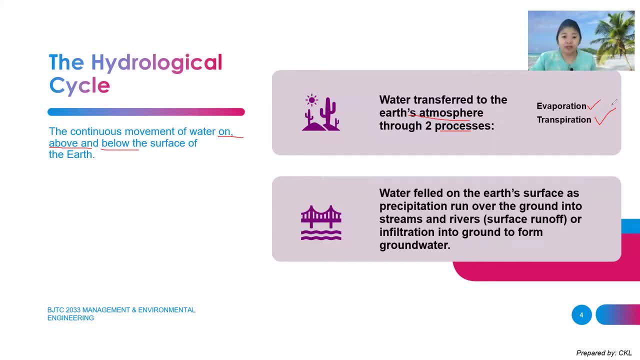 So the evaporations will be Happens Right. So the water fell on the earth surface as the precipitations. Why we call it as a precipitation, not rainfall? Because Precipitations means include snow In Malaysia. Yes, we didn't have snow. 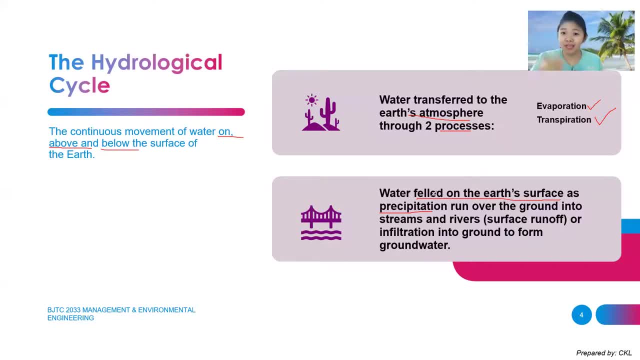 So most of you may be- Doesn't alert That some things that falling down from the top of the skies to the Surface of our earth Is actually- we call it as the general names- is precipitation, But then usually we only said rain. 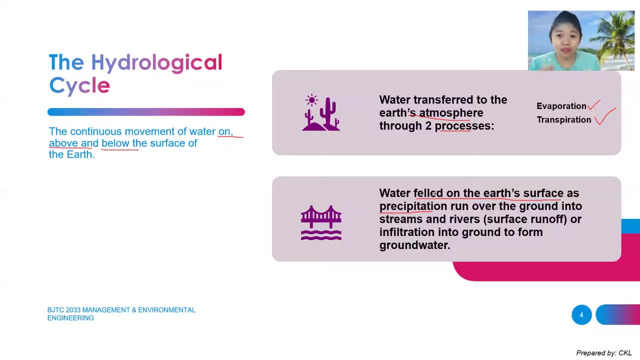 Rainfall, rain is dropping, Okay, But then you have to remember, for those have four seasons countries, They actually have snow, So the snow also being calculates, because one does snow fall down, It will melt, It will melt and become Water. 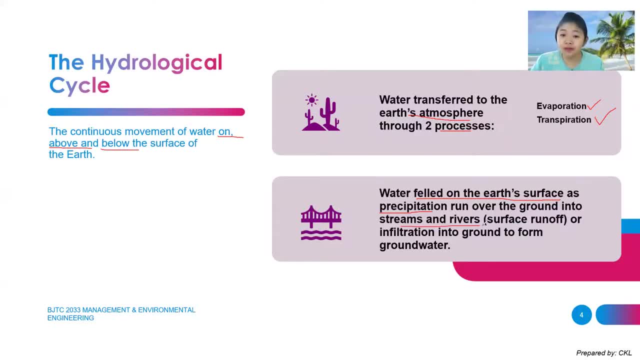 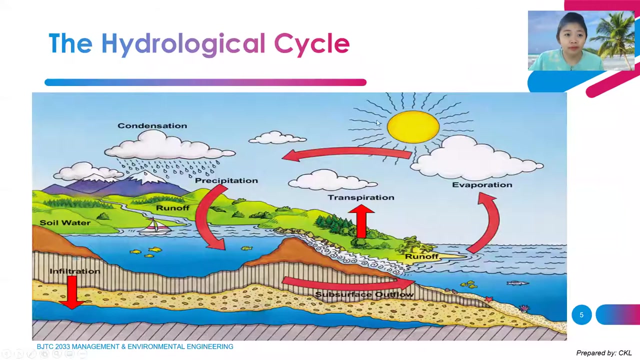 Okay, So run over the ground into stream and revolt, So we call it as the surface runoff- All infiltrate into the ground to from the ground Water. Okay, Right. So this is the complete image of the hydrological cycles. So from the first part, 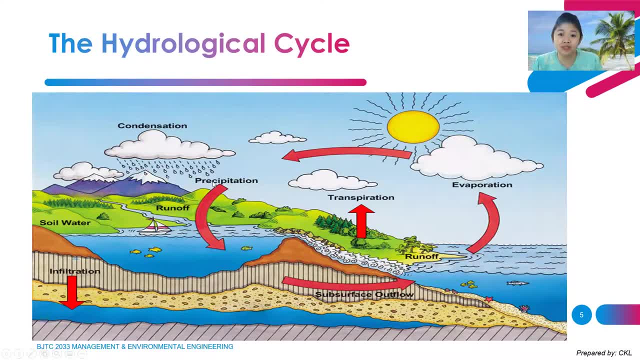 We will see Precipitations. This is the first process. precipitation When the drain drop, King, And the snows When the drain drop and the snow is falling down, So you will forms As the Surface runoff. Okay, 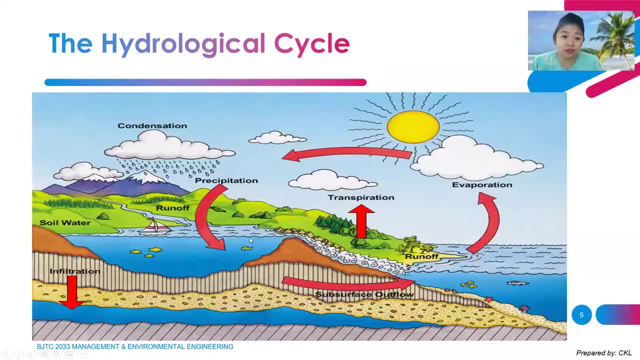 So when it come as the surface runoff, It will flow To the river Sea. Okay, So this is the lake. When sun is coming out, We will have the Evaporations And then transpiration means Those fogging. 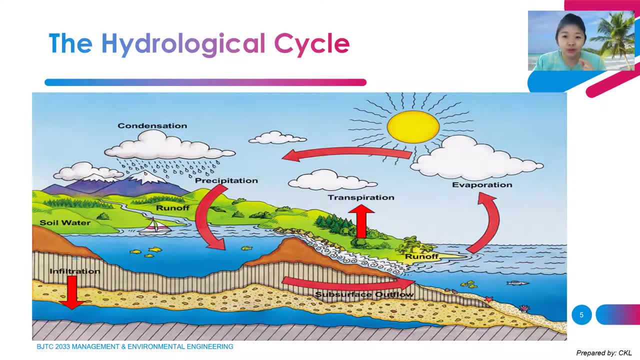 So okay, Last time, If you are, stay in, simple, You are in you. Every morning When you wake up, It's a very Blurry, So you have to fogging When the sun come out. So the foggings were gone. 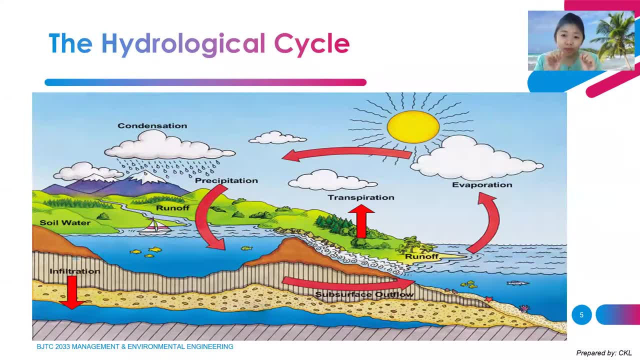 So the fogging is actually Those water molecules That having In our atmosphere. So the foggings Is actually From the Trees Or from the Air, Become Going up, Become the Cloud. So we call it. 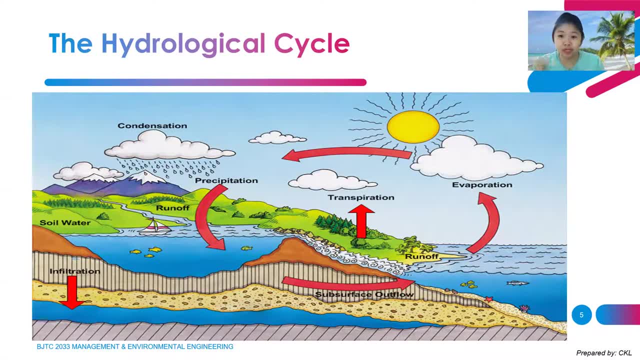 As a transpiration, Evaporations Means It definitely Will From the sea Or from the river, Is from something That on the Surface Okay. So after the Evaporations You go Up, There will be. 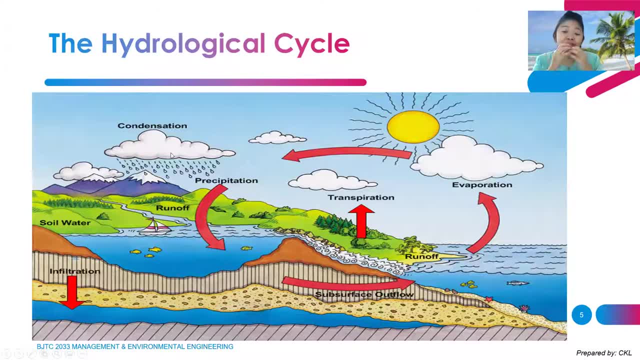 Condensations. You go Up, Then you will have The condensations. Everything's Will combine Bigger And bigger. The cloud Will become Bigger And bigger, Heavy And heavier, And then it will. 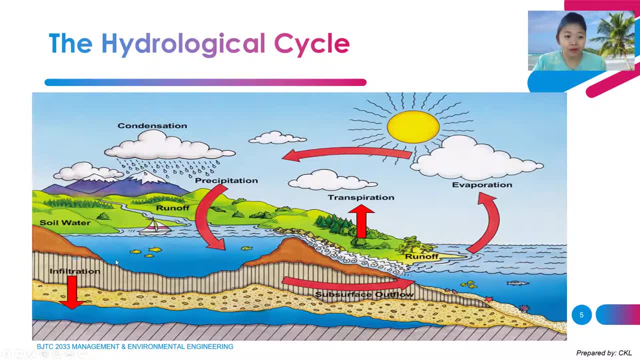 Drops Again. So once It drop Against We will return To the cycle As the Precipitation: Okay, Right. So once There's This, Those Land That not Concrete, So the 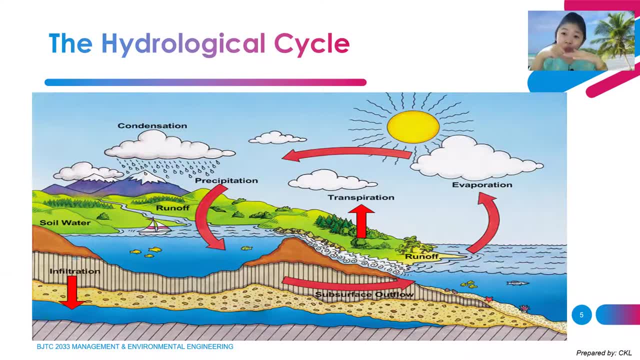 Water Can Penetrate. It's Like A sponge Water Can Go In. So when The Waters Go In, It Means It Become The Infiltration. So 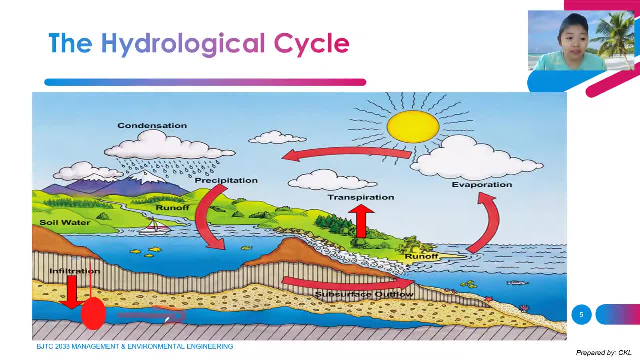 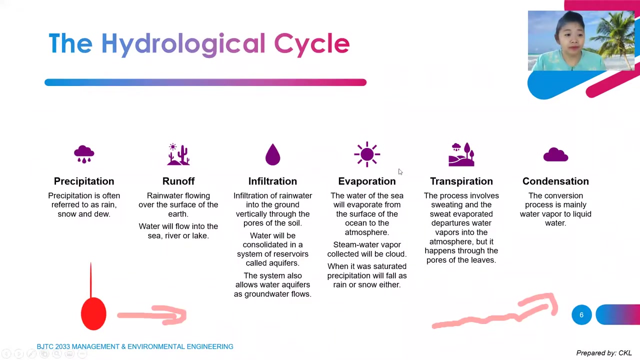 What The So It Will Forms The Underground Water For Us. Okay, So Here Is Our Underground Waters, And Then These Underground Water, If There Are. 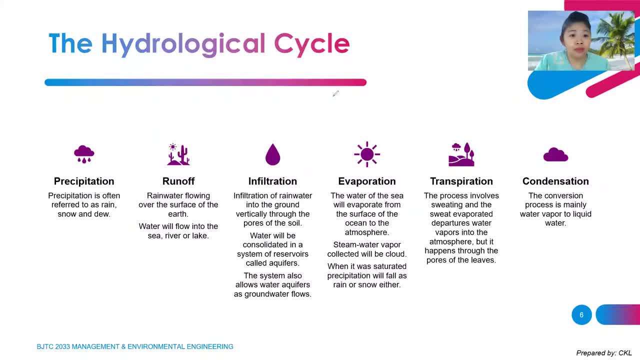 Some Cracking Here. It Also The Explanations For Each Process. First We Have The Precipitations. Rain Is Dropping, So Precipitation Is Often. 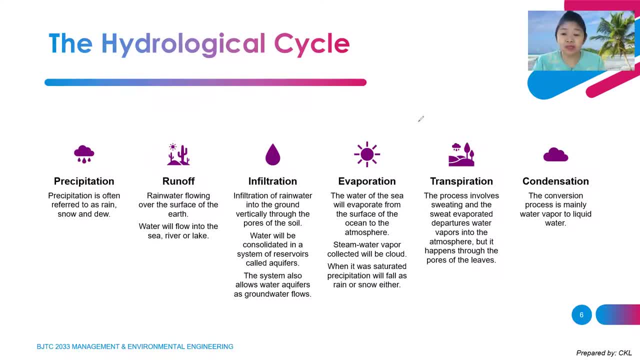 Referred Often Referred To As Rain, Snow And Dew, Okay, And Then Hold On, Hold On, Hold On, Okay, Sorry, Continue Valley, Okay, Right. So 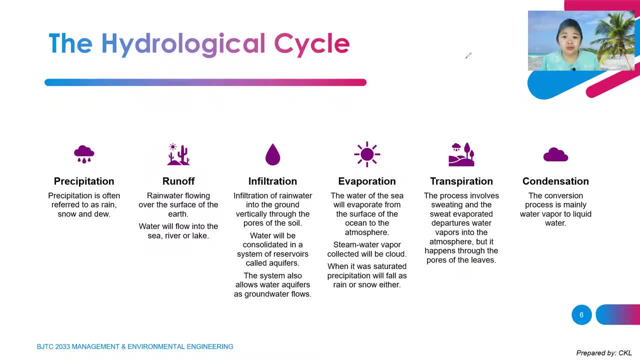 So Evaporations Means When You Having The Suns, All The Waters Will Go. Evaporates From The Core Of The Leaf. Okay, Usually Is The 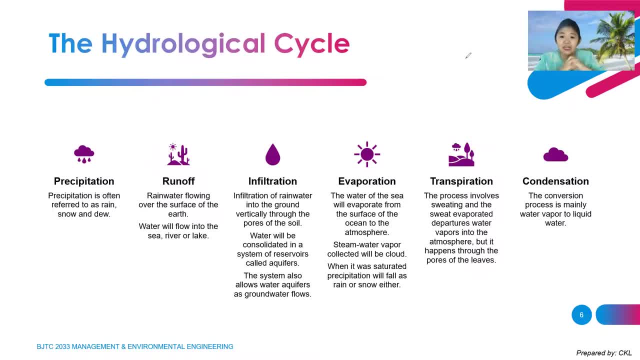 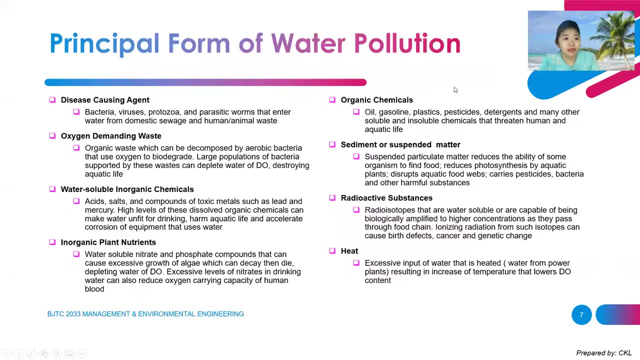 Drops Of The Leaf On The Leaf, And Then, Finally, Is The Condensations, Where All The Small Drop That Been Evaporates. When You Understand, 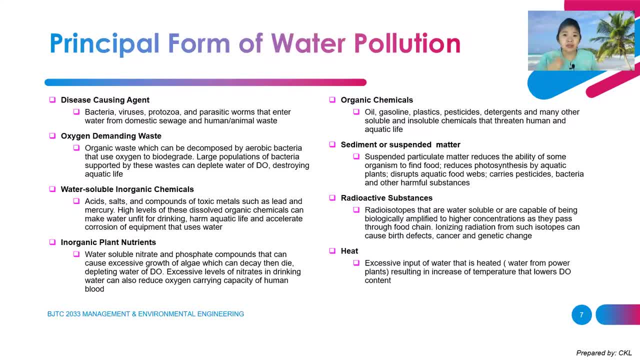 The Concept When You Understand The Hydrological Cycles, How It Happens. Not Now, We're Moving Forward. So When We Talk About Water Pollutions, 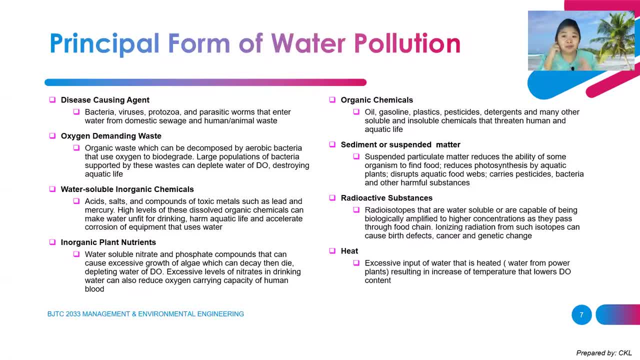 How We Identify This Pollution Cause. That Can Cause The Pollutions, Can Be The Agents For The Pollution. The First Thing Is Actually The Disease. 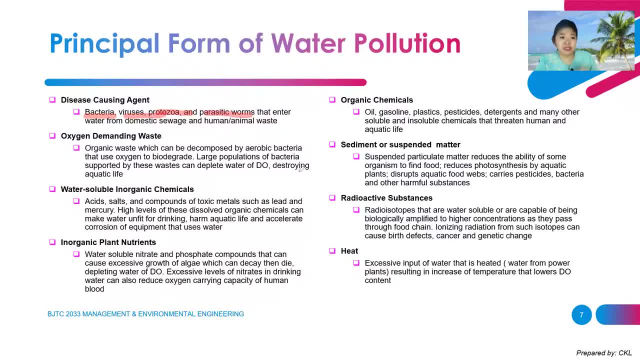 That Causing Agents. So You Will See Here. Second Is The Oxygen Demanding Waste, So The Organic Waste Which Can Be Decomposed By The 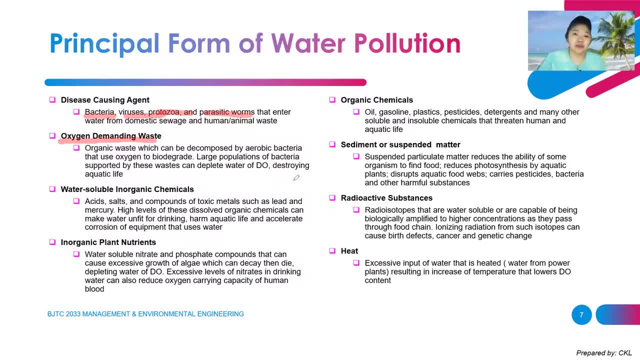 Bacteria By You That Using Oxygen, So When The Large Populations Of The Virus, So It Have To Be Some Things, That Virus Or Bacteria. 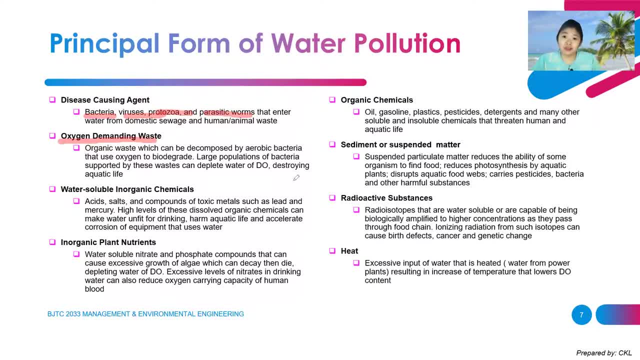 So If You Having Like The Precious Site Of Worms So Where It Comes From The Domestic Toilet, Your Toilet Might Be Attached On The 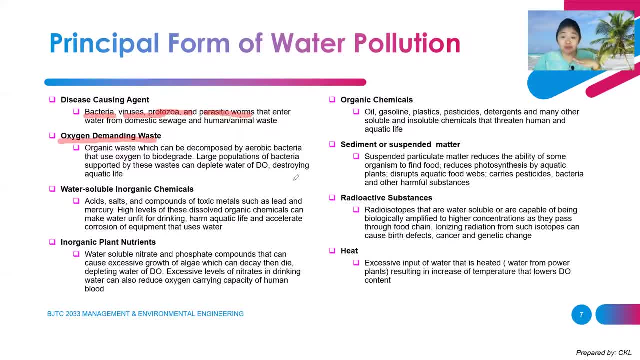 River. So When You Doing Your Business It Will Directly Go To The River. So This Kind Of Waste, Those Things All Get Into The 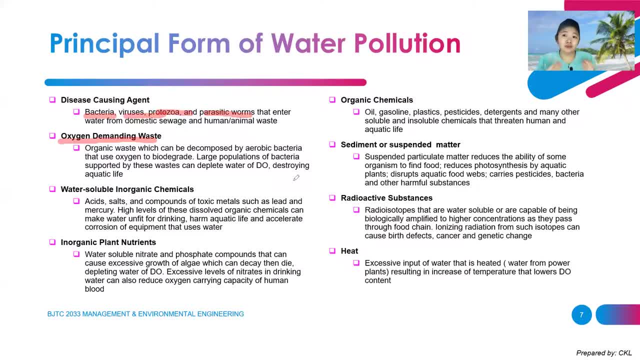 River. So Here Is The Place. So When You Just Imaging If Those Waste Being Go Into The River And Then You Drink The Water From, 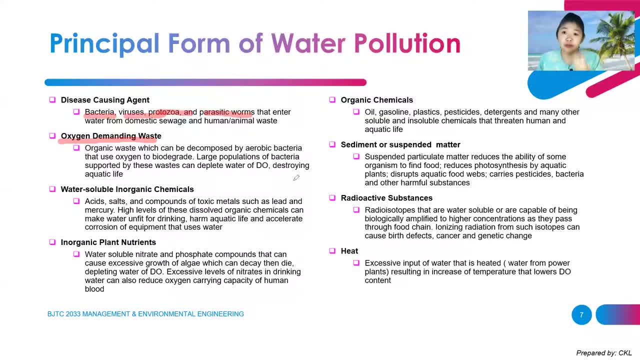 The River. So If You Have A Micron Of Plag Tons, So If They Will Grow, But There's One, If Your Populations They 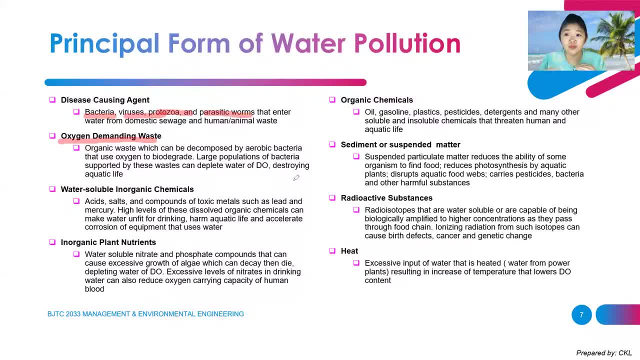 Grow Too Much, So What Will You Have? Too Much Of Oxygen. So When The Fish Die, So Our Waters Is Become Like Polluted, Because. 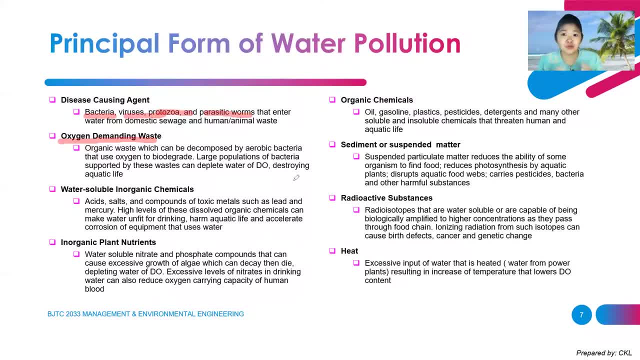 If You Having In A Big Amount, So It Will Be Low Fish, So The Oxygen Will Be Taking Take Over By The Plag Tons. 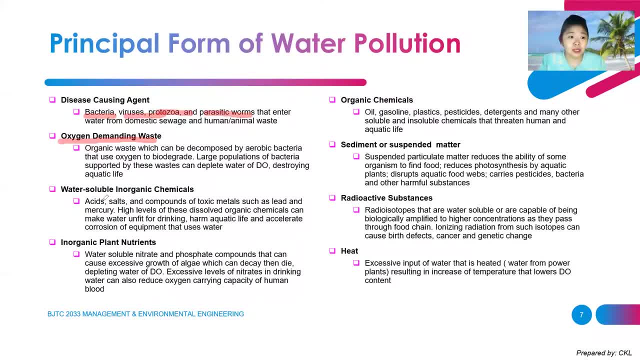 So When The Oxygen Take Over By The Plag Tons, So It Will Be: If This Thing Can We Eat, This Thing We Cannot Eat. 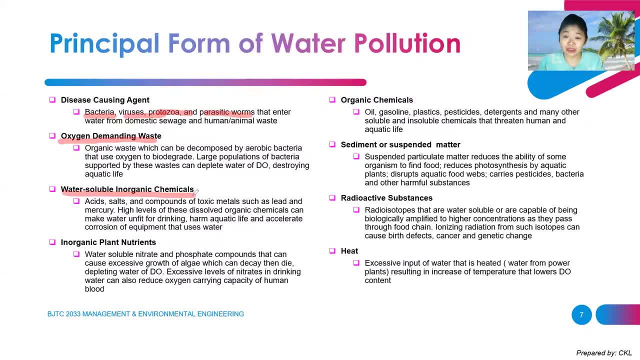 As A Human, We Cannot Eat. So If This Been Put Inside Our River? So What Will Happen? Our Phosphor, Our Fertilizer Or 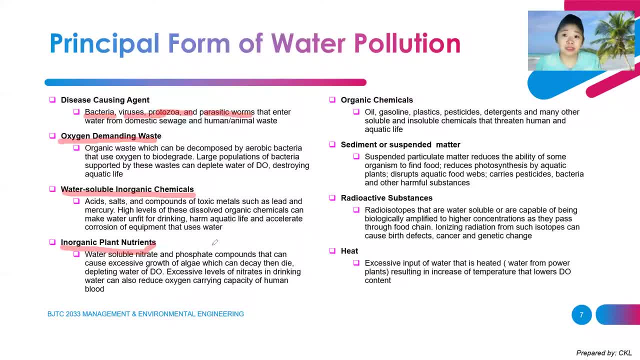 Even The Pesticide Killer. Okay, So This Also Will Depleting Our Dissolve Oxygen. Number Five Is Organic Chemicals: Oil, Gasoline, Plastic, Pesticide. 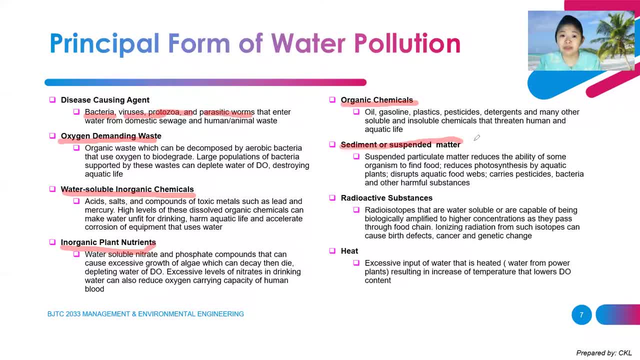 Detergent Attracts The Ability Of Some Organism To Find Food, Reduce The Photosynthesis By The Aquatic Plants. Okay, Inside The Rivers We Still. 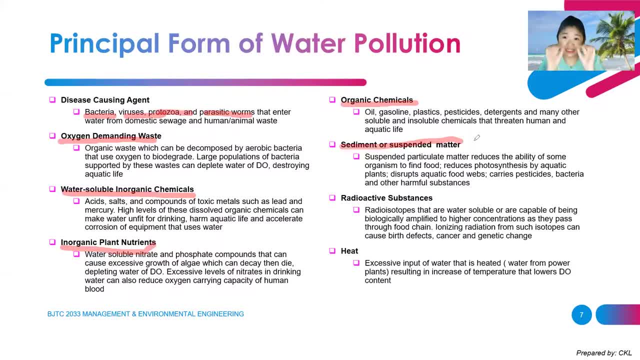 Have Plants, They Will Still Produce And Doing Their. It Cannot Go Through, So Photosynthesis Cannot Be Done. So When There Is No Photosynthesis, So 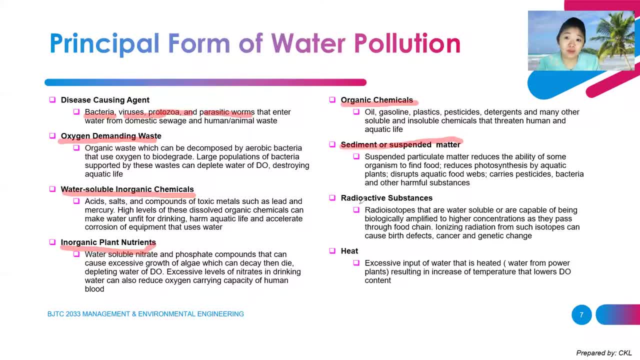 It Will Full With Carbon The Outside, So You Didn't Have Any Oxygen Or First No. Radioactive Is Something That Definitely Won't Be Good. 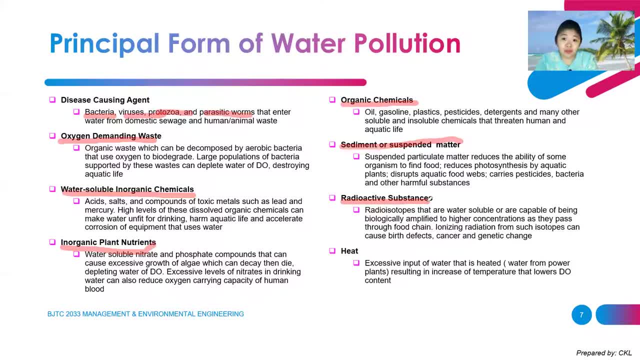 So Even Is The Same. So These Cases Are Also One Of The Example That You Can Relate To The Nuclear, Because All The Water 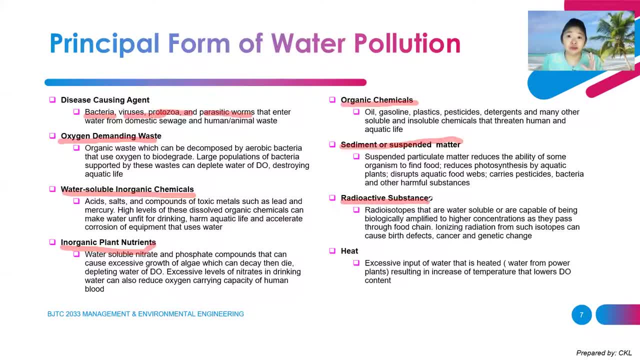 That We Clean Up The Nuclear Been Released To Our Oceans. Okay, So This Is Something That We Need To Know. Finally, Any Living Organism- 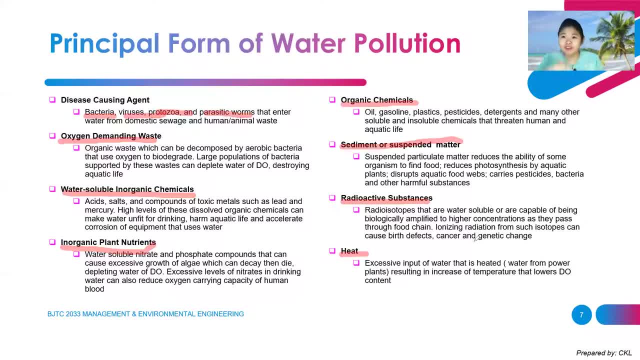 In The Waters. They Also Don't Like A Hot Water. You Put A Fish Inside The Hot Water. Can They Survive Or They Will Die. 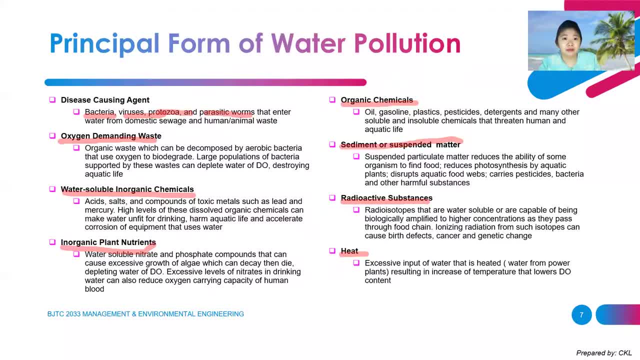 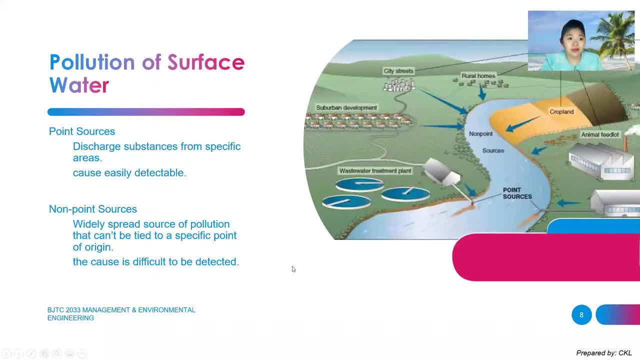 So We Have To Clean Our Oceans, Right, Okay, Okay, Okay. So You, At Least You Have The Basic Ideas When We Say Some Things. 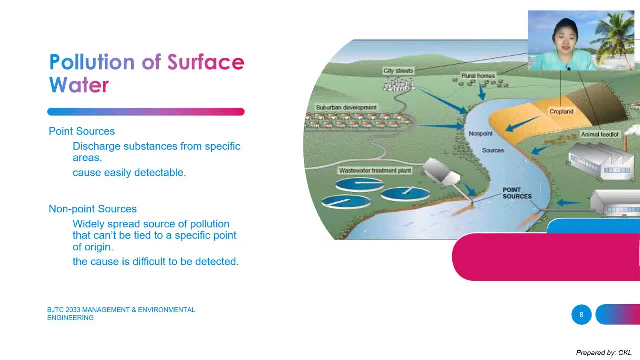 You Are Doing Pollution. You Are General. Now We Look Into Specific. First. We Look Into The Surface Water, Where We Call For The River. So 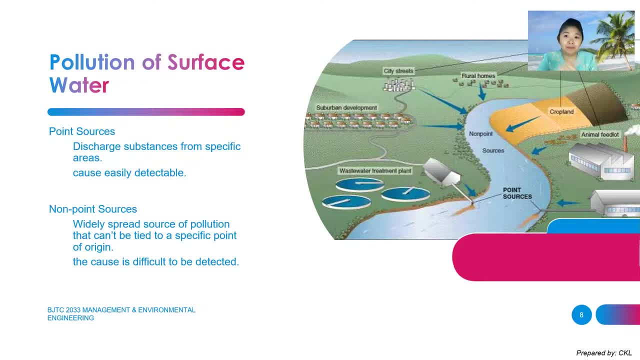 The Pollution Of The River. Pollution Of The River You Can Identify, You Can Detect Is Coming Directly From A Specific Areas. So From This, 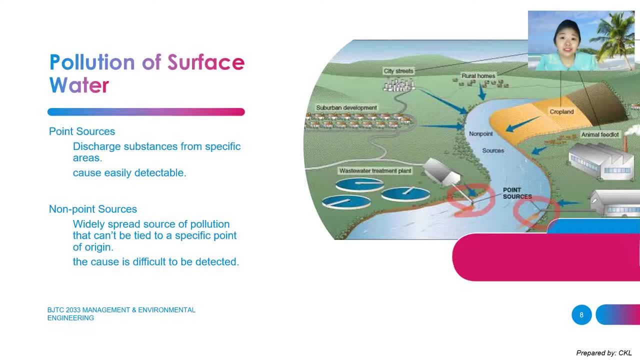 Figure You Can See. This Is Point Source. This Is Point Source. That Specific, Specific Point, The Where Is Come From, Is Very Hard For Us. 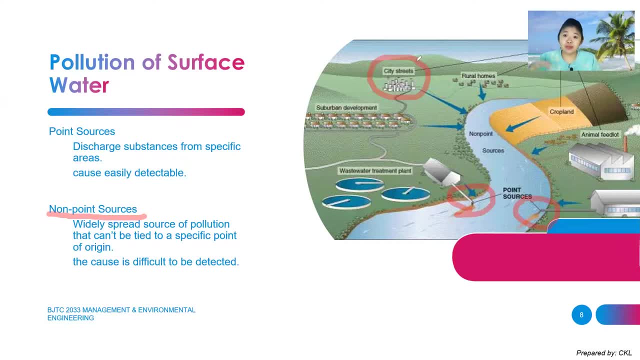 To Identify. So, Such As Example: When You Have A City Street, You Are Walking On The River. Is Will Actually Become The Sediment. Okay. 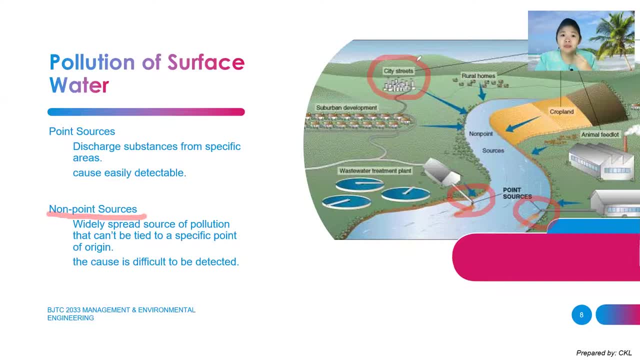 So This Is A Non-point Source. That Means When We Talk About Non-point Source Is Something That You Don't Know, Where You Have A. 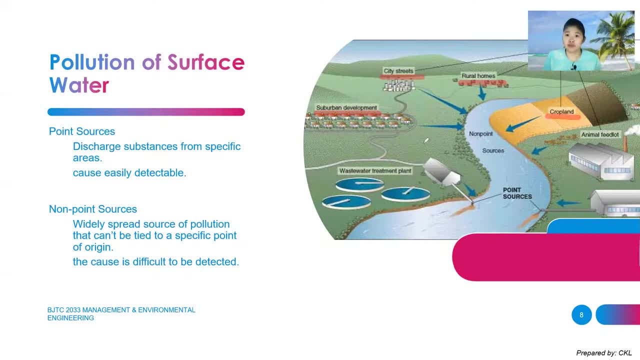 Piece Of Land. You Say, Okay, I Want To Do Something, I Want To Do Some Development, So I Cut All The Tree First, Okay, So 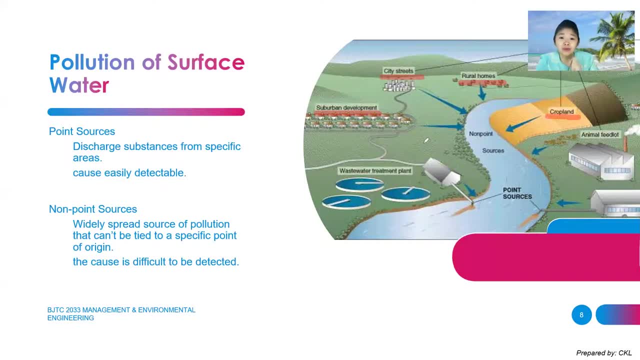 This Is Something That You Can't Identify. You Can't Really Know Where Is Come From, Compared To The Wastewater Treatment Plants, Because You Have 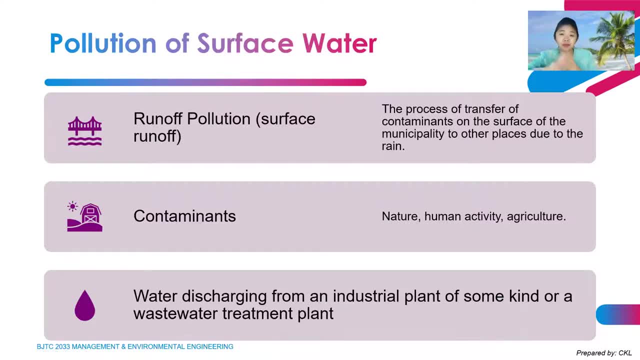 The Piping, And Usually The One Point. So This Is The Two Main Categories. So From These Two Main Category There Are Three Types Of 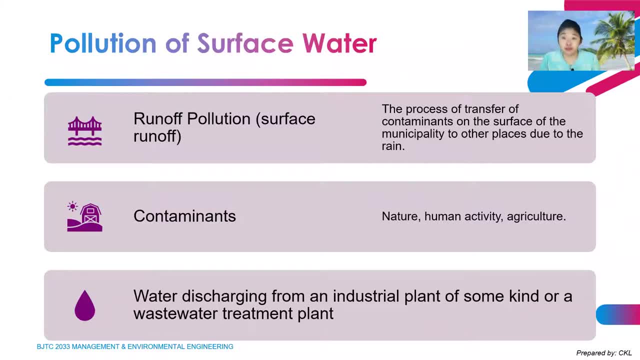 The Pollution. The First One Is The Run Of Some Things. The Water Will Flow Along, So We Will Go Through Along Until The Reverse. Okay. 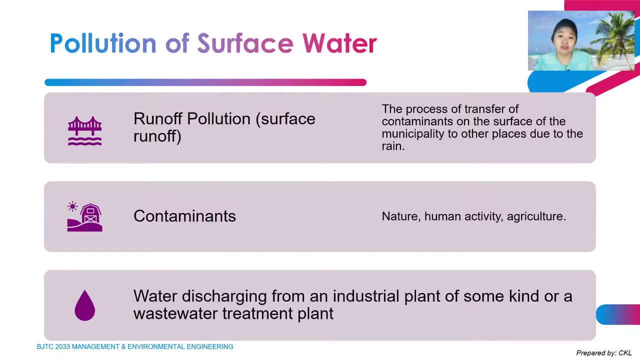 Second Example: If You Still Remember, I Think Maybe Only Those New Students, Okay, So That River Usually When There Is No Raining. You Will. 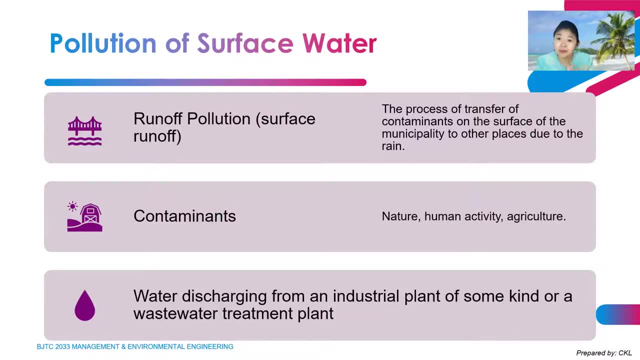 See, The Water Is Quite Clear, But That's When There Is Raining Season The Water Become Like We Actually Have The Sand Mining, So They 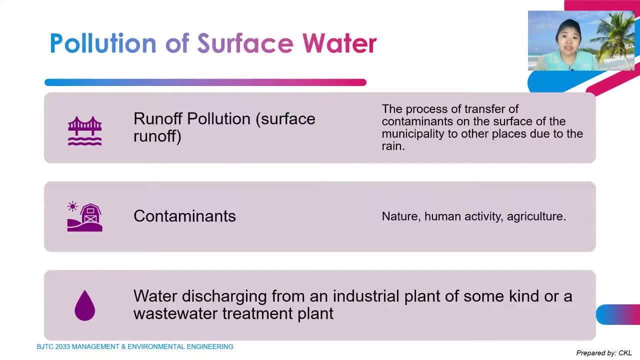 Have To Clean The Sand From The Mountains That They Take, So All The Waters Will Be Coming Through. And Then The Natural Activity Or Agriculture. 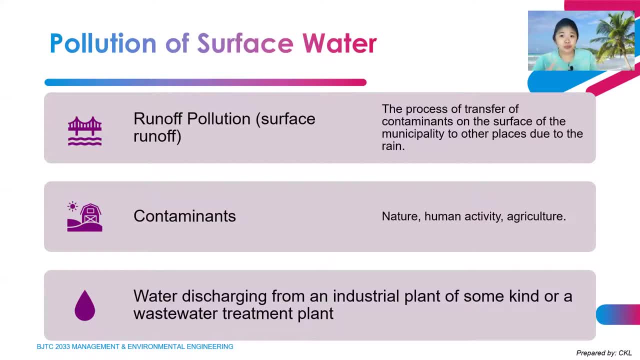 Is Usually Include The Fertilizer, Our Pesticide, So You Might Be Curious How The Fertilizer Will Impact, Because You Put The Fertilizer. 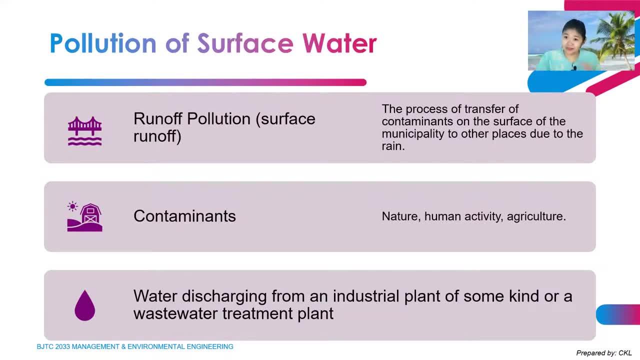 In The Water Fertilizer. If There Are Wind When You Spray Something, Will It Bring Through, So It Will Fly And Drop It On The 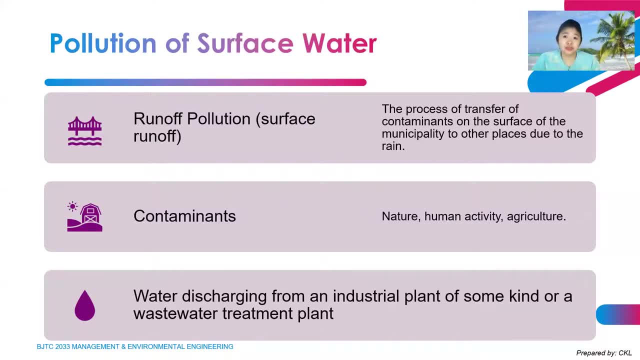 River. Okay, So The Final One Is That Doing The Industrial Works And Then They Didn't Sense The Water To The Wastewater Treatment Plants. 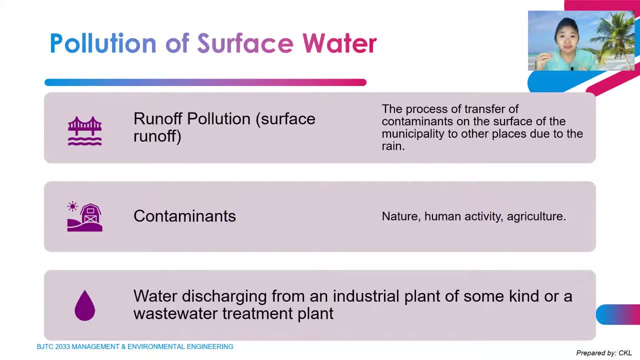 But Then They Discharge Directly, The Most Easier To Be Traced. Why Factories? Yeah, Today You Have, You Die. Your Coat Is A. 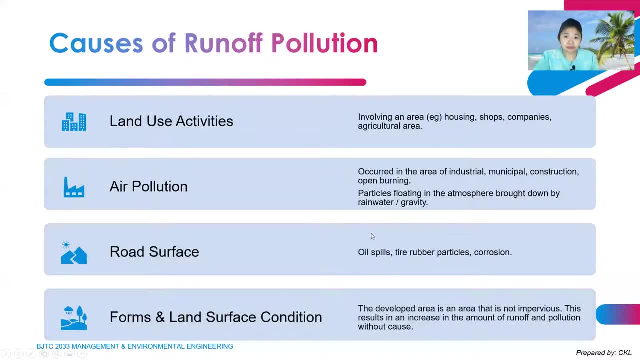 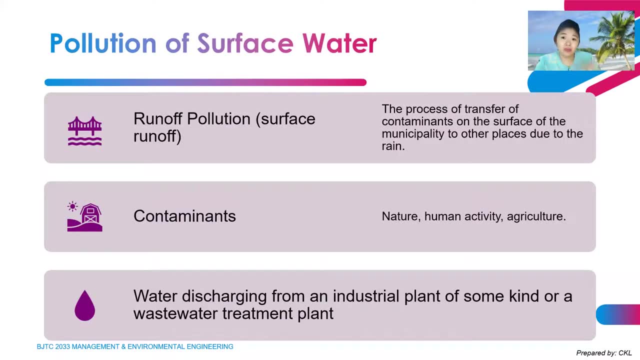 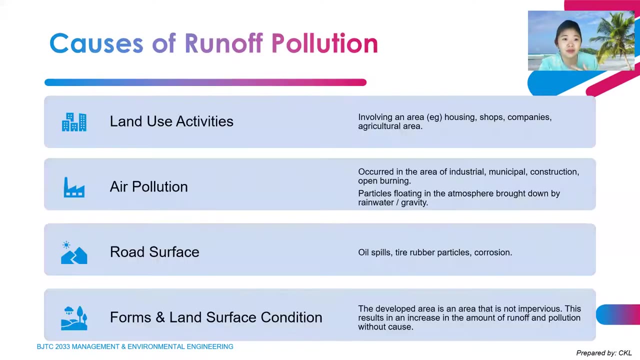 Red Color, So Tomorrow Is A Blue. So This Is Something That The Pollutions Of The Surface Water. Now We Having Like More Details. One. 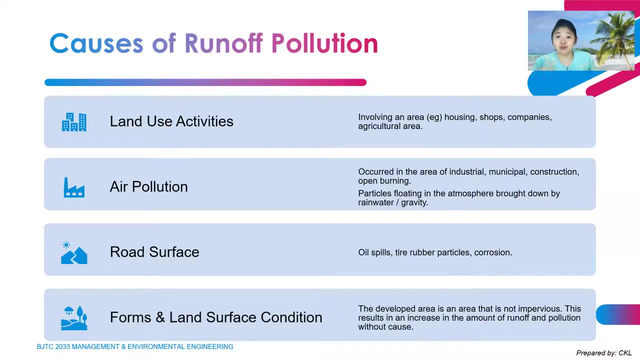 So What Is The Run Of Pollutions? So First Is The Land Use Activities. When You Are Losing Your Housing, Your Shops On The Surface, 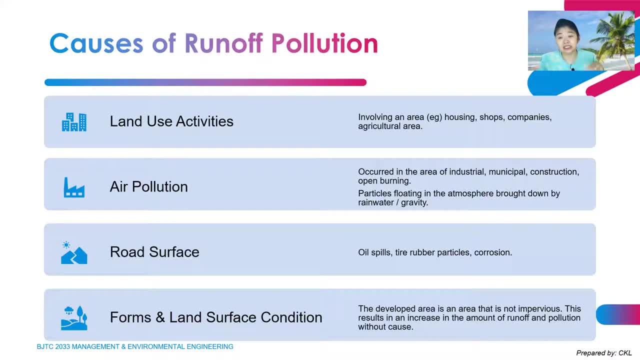 It Will Go Through With The Water. It Will Flow Along Jalan Skully. Okay, Some Time Until The River. Second Is The Air Pollutions. 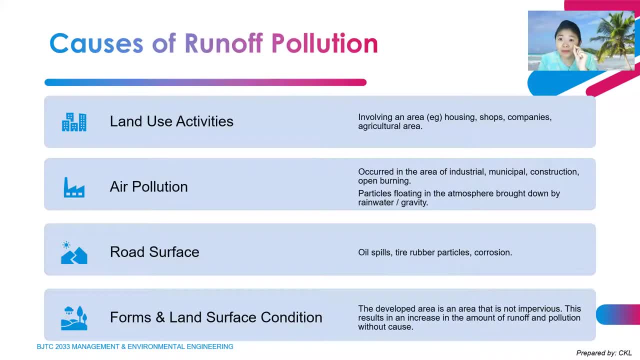 Okay, Have. So. Means Is A Small Particles, So When It's Going Up, A Small Particle, When There Is Raining, The Rain Will Bring. 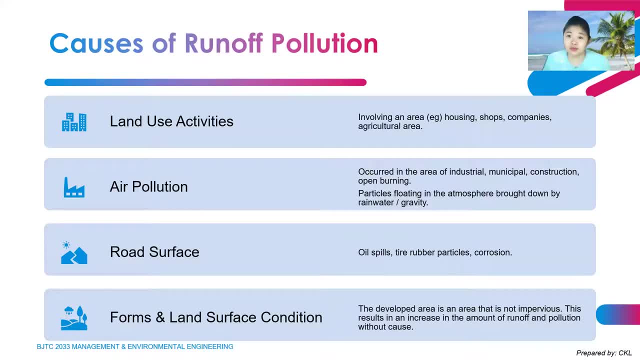 It Back To The Surface. Okay, So Open Burning. So The Particle Floating In The Atmosphere Brought Down By The Rain, Water Or The Gravity? 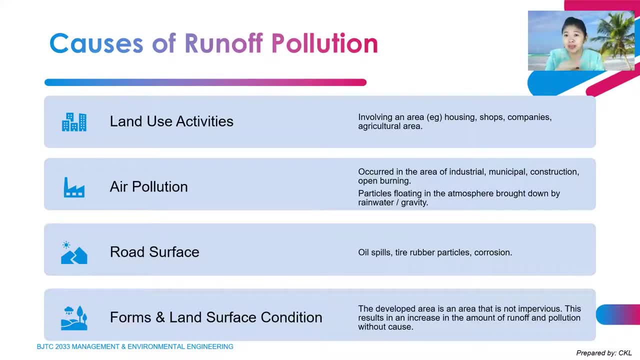 Okay, So On The Road Surface Sometimes We Have The Oil- The Rain Is Coming. Where Will This Go? It Will Go To The Small Stream. 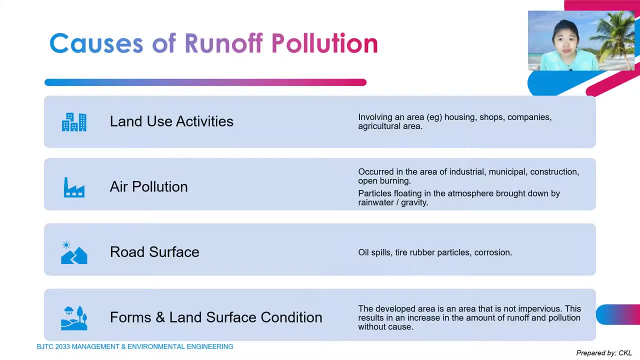 Long, Long And Because Loud, So It Will Go To The Small Stream Beside To. This Is Not Impervious, So This Result In An 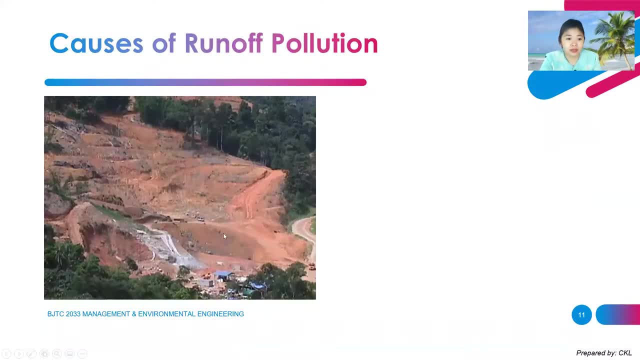 Increase In The Amount Of Runoff And Also Pollutions. Without The Cost King, I Will Show You The Photo For Flow Through, So You Will. 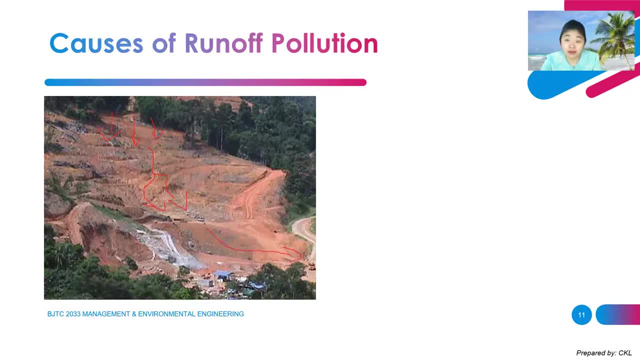 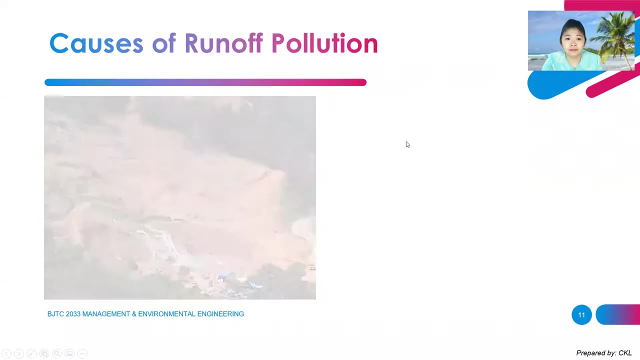 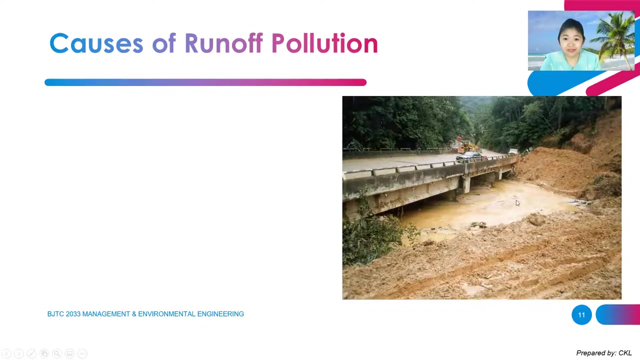 See, This Is The Mark, So The Waters Will Go Through And It Will Go To. This Is The Road Coming To The Road. This Is: 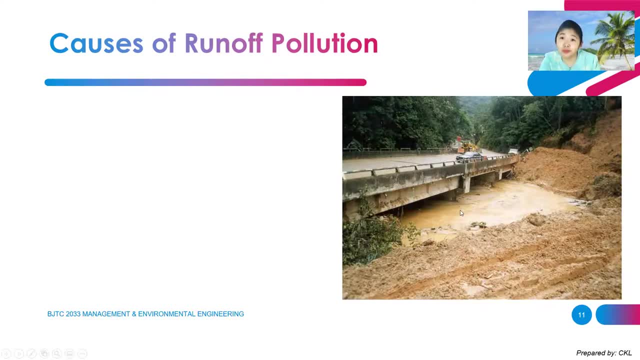 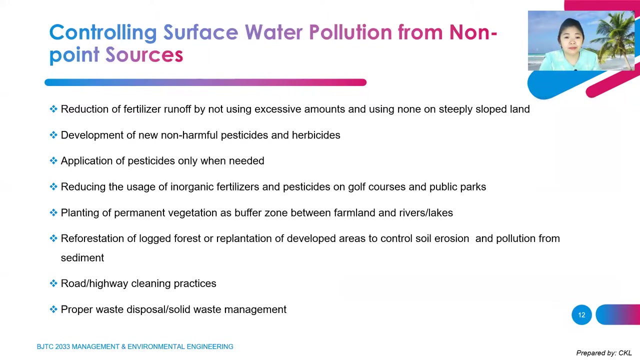 The Color. So Do You Think This Is Kind One, One Of The Pollution? So What The Pollution? It Doesn't Mean When You Throw Your. 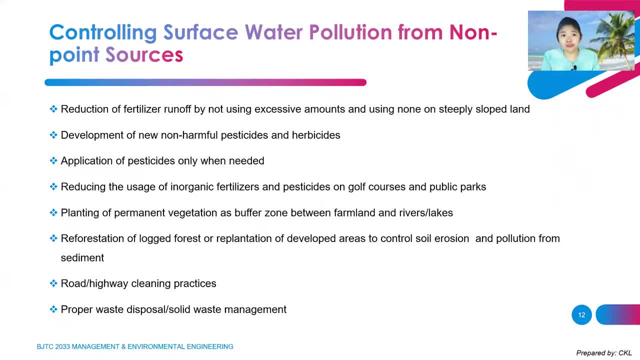 Rubbish Inside The Water. So Control This Surface Water Pollution From The Non Point Source. So First We Have To Reduce The Fertilizer And 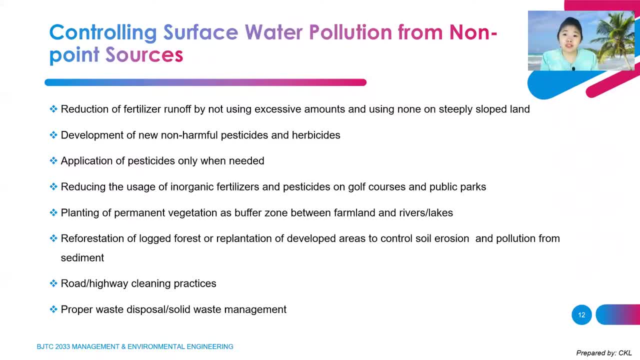 Then We Have To Develop The Non Harmful To Our Environment. Okay, Plant The Permanent Vegetation As The Buffer Zone. So We Put Some Plantations. 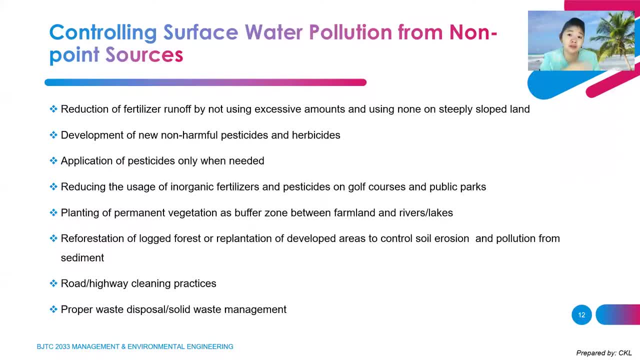 So When The Rainwater Bring It Down At Least, That Is Something That. And Then Reforestations Of The Log Forest, Those Tree That You 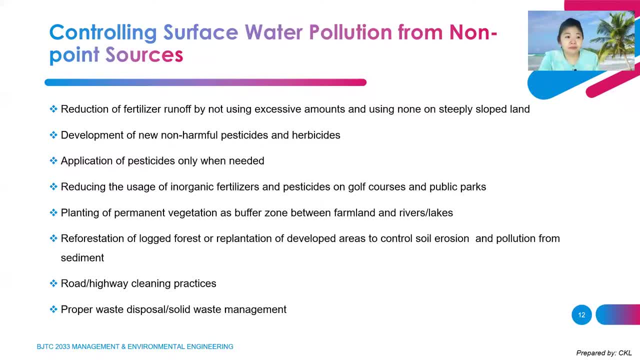 Been Cut, We Have To Replant Okay, So That It Won't Be Bought Okay Road Or Highway Cleaning Practice, The Proper Waste Disposal. So 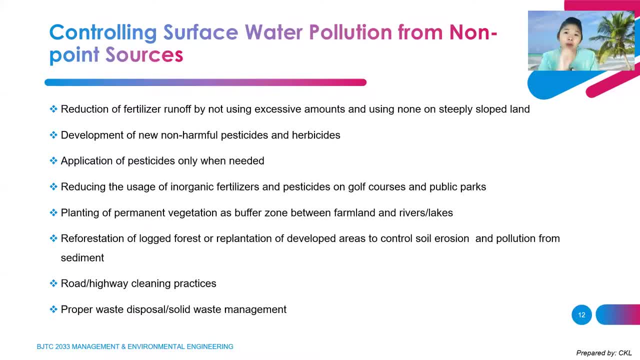 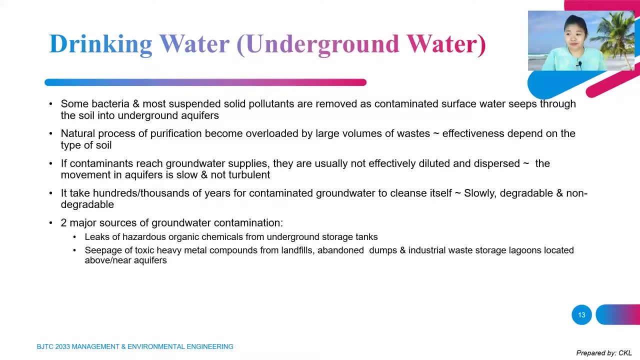 The Solid Waste Management. So You Will See, Is Actually Relate. The Whole Is Not Only From One Part. Okay, Right, So Next Is To 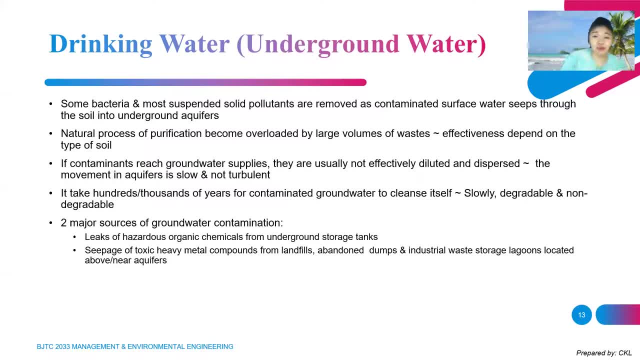 Take Care. Okay, If These Become Polluted, Even Worse. Okay, So Some Bacteria And Most Suspended Solid Pollutant Are Removed And The Contaminant 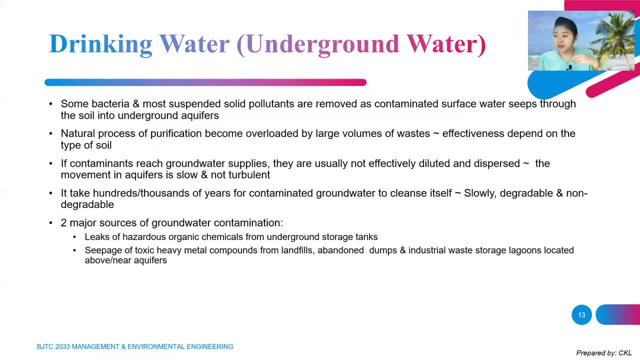 Surface Water Sip Through The. I'm Not Sure. Have You Ever Tried? I Will. I Can't Do It Now, Okay, So I Will Give. 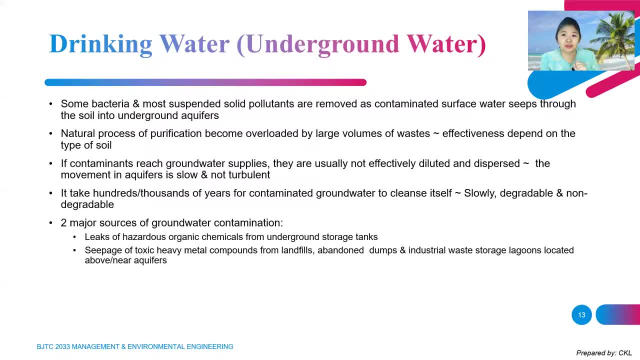 You The Videos You Can See. So When You Have These Filtrations Is Actually Been Help Us To Clean Our Waters. So That's Why. 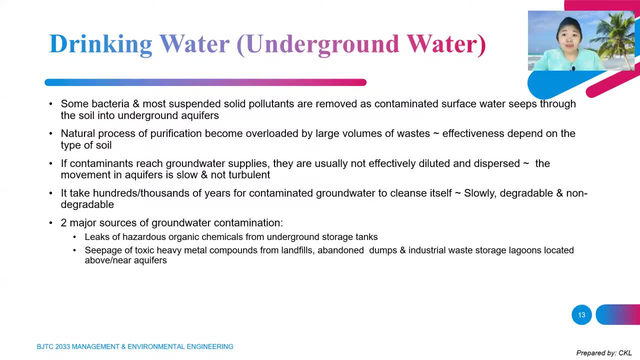 Is It When It Sip Through The Side? So The Nature Process Of The Purification. So If The Contaminants Reach The Groundwater Supplies. 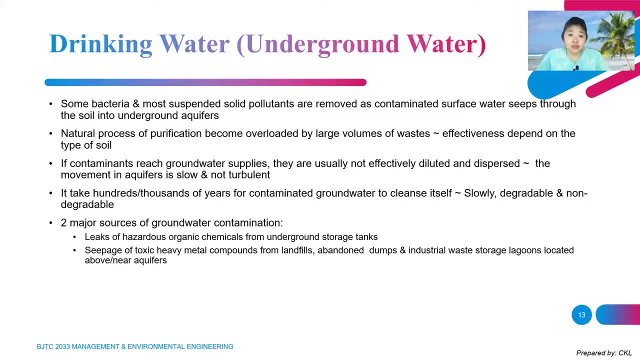 They Are Usually Not Effectively Dilute Or Disperse Because The Movement In The Aquafire Is Slow And Not Turbulence, So It Will. 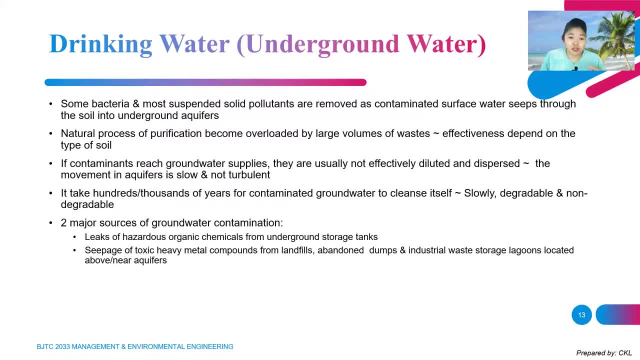 Cause Our Groundwater Become Polluted. Okay, So First Is The Lick Of Hazardous Organic Chemicals From The Underground Storage Tank. This Is Actually 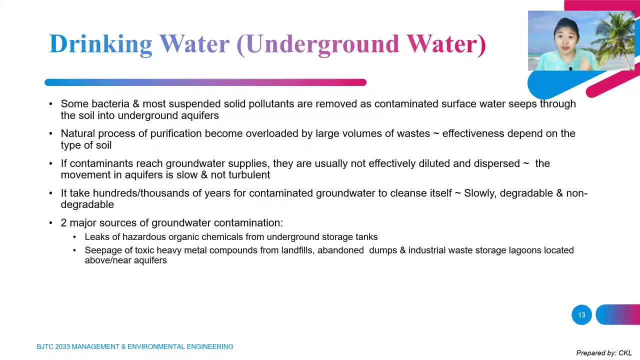 From The Landfill, Those Rubbies That Will, So Those Things Will Go Into The Water, Our Underground Waters. Okay, First Thing. Second, When You Buy, 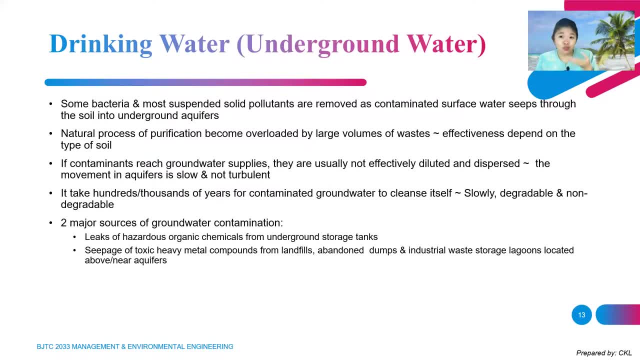 A Rice And Then You Didn't Finish It, You Left It, You This Thing. After Some Days It Will Become Like Wet And Liquid. So 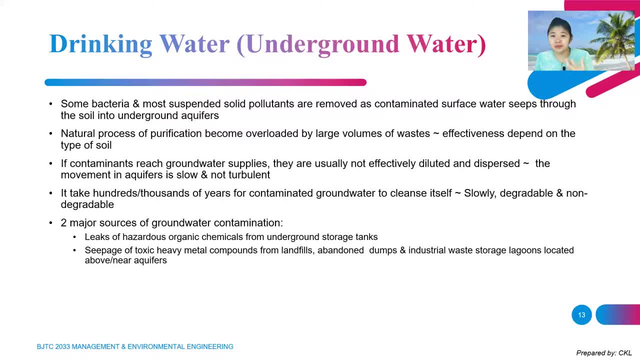 These Liquids Will Infiltrate To Our Underground. So If We Didn't Well Manage Our Solid Medicines, If You Didn't Finish Your Medicine, Have 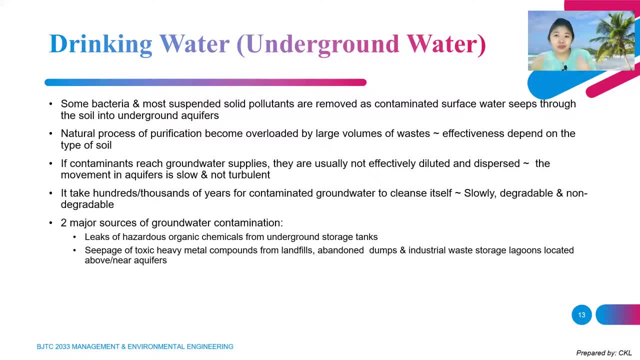 You Ever Return Back Or Go To Hospital And Dispose It In The Box? No, Nobody Right, You Will Just Throw A Rainfall, So What? 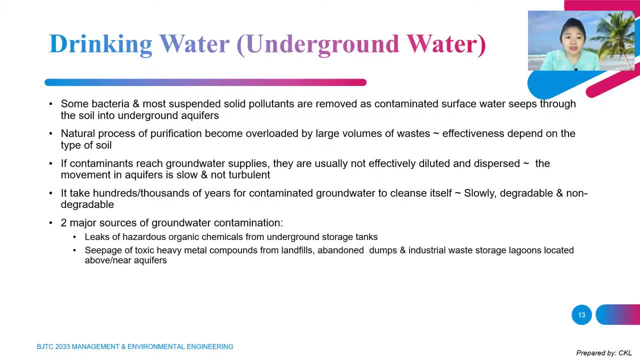 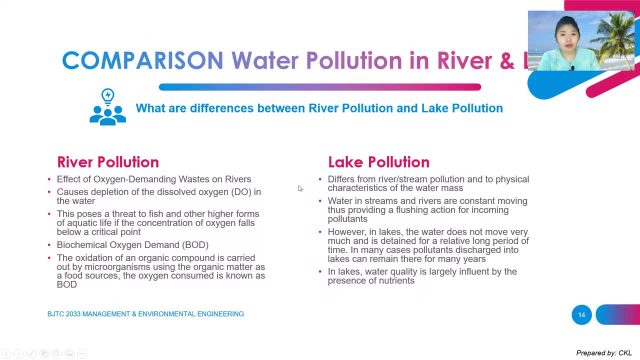 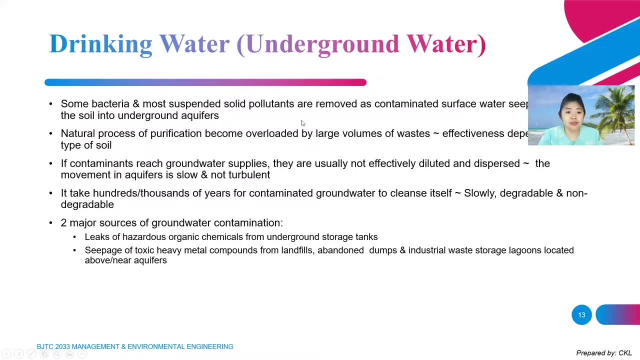 Happens Is Still The Infiltrates To Our Underground Water. Okay, So Next Is The Toxic Heavy Metals Compound From Landfills Abundant Dumps. 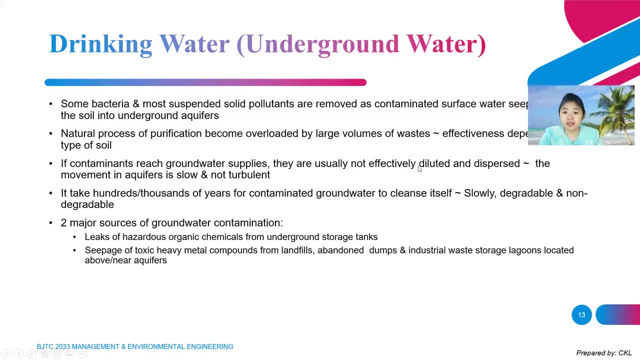 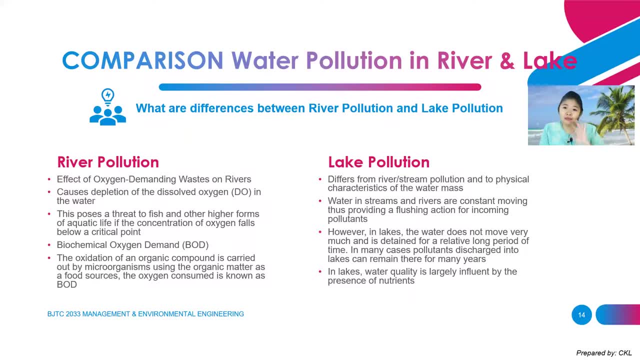 Or Industrial Waste And Because It Cannot Be Dilute Or Dispersed. Okay, So Now I'm Showing You What Is The Difference When We Say: 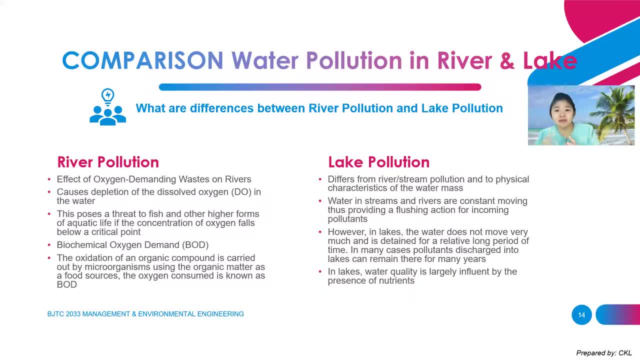 About The River And The Lake Management. Okay, The Comparison Is Like The River Pollutions: It Will Effect On Our DO, So Our D Soft. 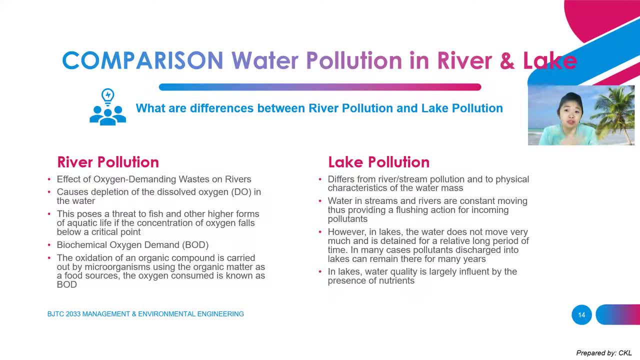 Oxygen Will Be Become Low. So This Will Pose A Trick To You: Drop Something Here. It Will Keep Moving. Okay, Let's Say You Drop. 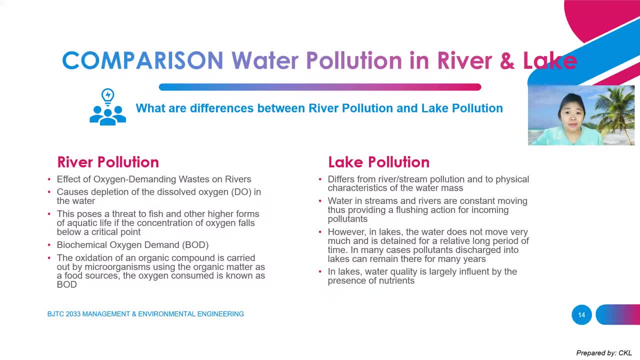 A Dye Color. Okay, You Drop A Dye Here And Then The Rivers Will Move. So During A Bottles, You Drop A Dye Inside. 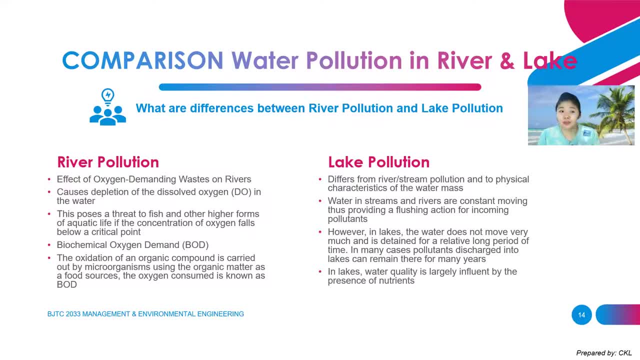 It Will Only Pollute The Whole Bottles And That It Won't Go Anywhere. So This Is The Difference Between The Lake Pollutants, However. 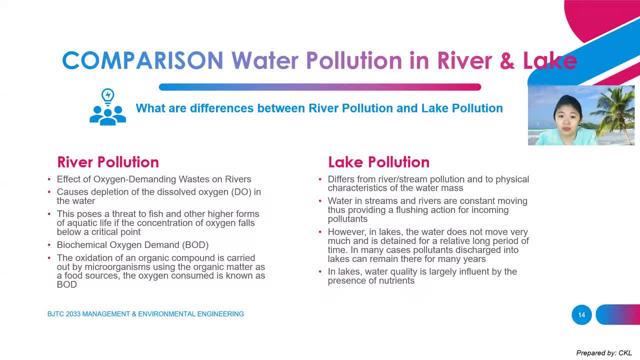 In Lakes Or Underground Waters The Water Does Not Move Very Much, So It Will Stay There Relative Very Long Period. So The Discharge So 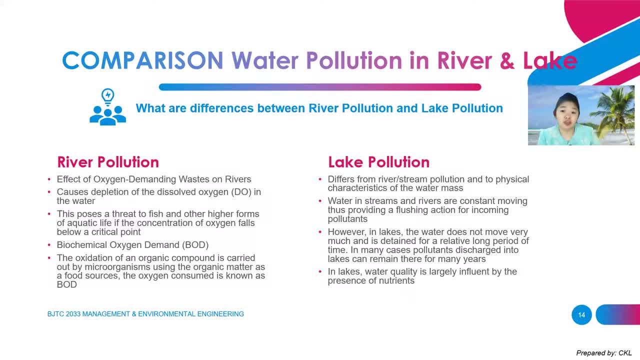 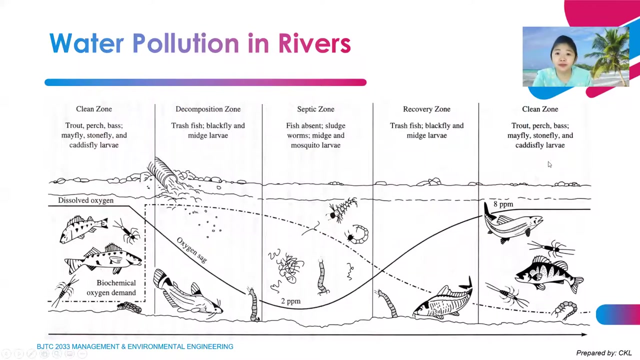 Therefore The One Is Keep Moving So It Can Be Dilute, Okay. Second One For The Lake Pollutions: One It Enter Is Will Be Stay. 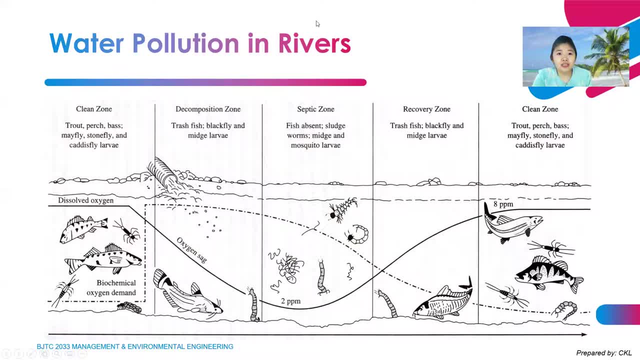 There For Long, Long Times. It Will Recover Back To The Normal, Unless The Oxygen Is Going Down. But Then After Some Times It Will Recover. 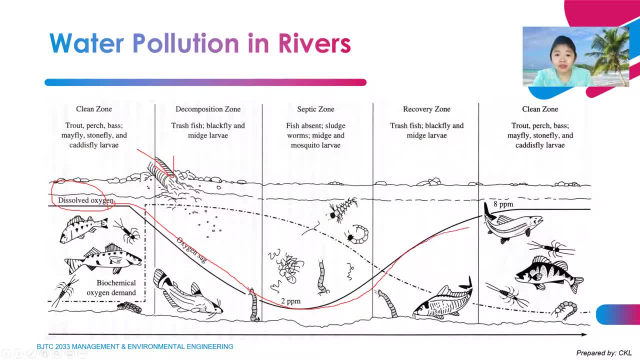 Back To The Normal, Unless The Oxygen Is Going Down. You Have Pollutions Here. You Have Pollutions Here. You Have Pollutions Here. Then It 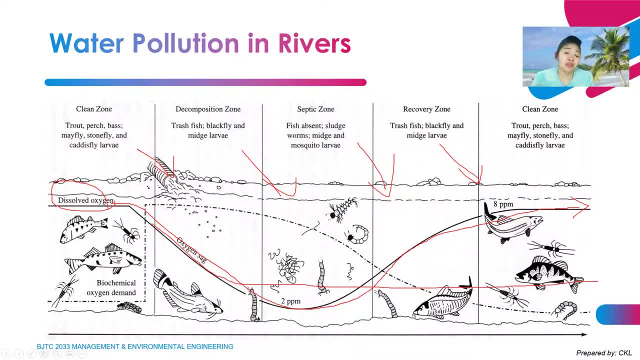 Will Be All The Times Very Low. Okay, So This Is The Difference, The Rewards. Do You Have Time To Clean Up? No, So It Will. 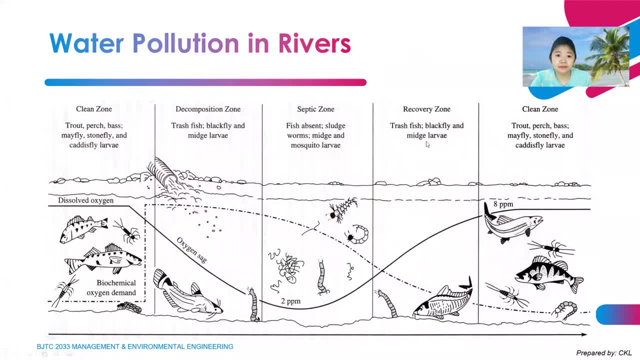 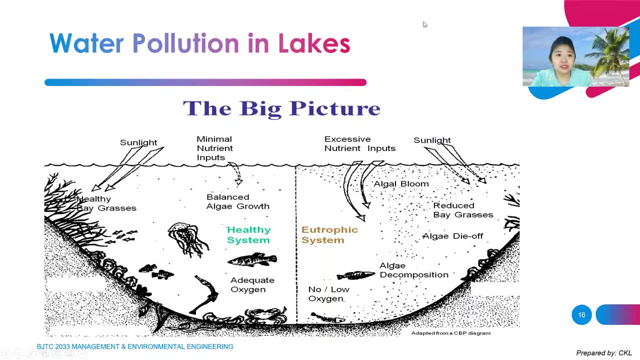 Become A Polluted River Right. However, Compared To The Lake, You Will See, Is A Totally Different. So It Will Stay Here, So You Will. 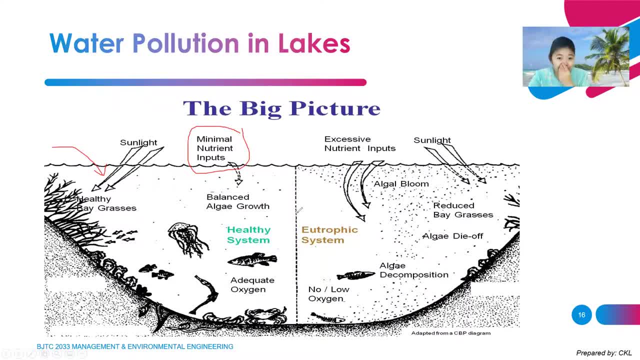 See If This Is The Healthy System. We Only Need A Minimum Nutrients Input. But Okay, So The Nutrient Is Actually The Oxygen, So The 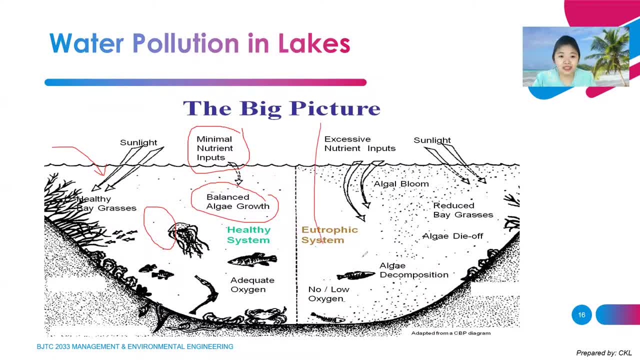 Oxygen Also Will Be Enough. If It's Not Much, Okay. But You See, This Is On The Another Side. You See, This One Is Not. 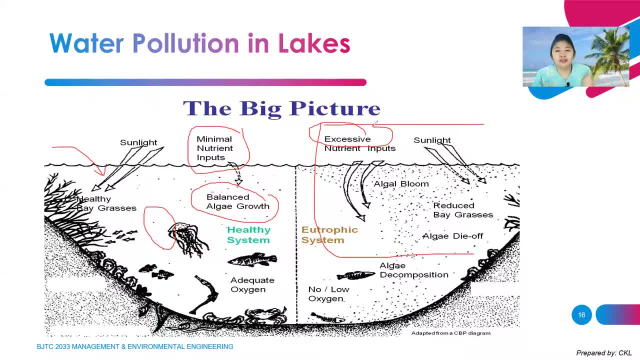 The Nutrient. You Think, Oh, I Feel I'm Weak, I Need A Lot Of Vitamin, So I Eat A Lot. Then You Become Overdose. 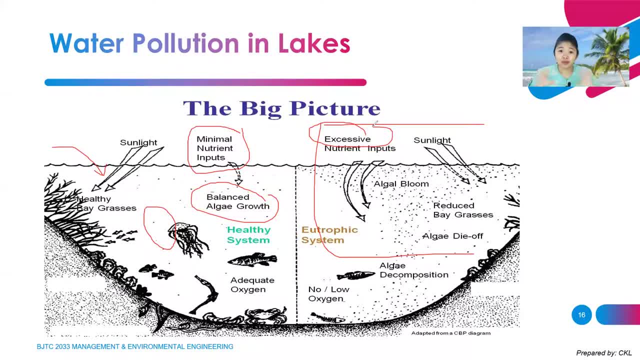 It's Actually Not Good, So It's Okay. And Then When You Have Too Much Of Organism Inside, The Oxygen Level Will Become Low. So 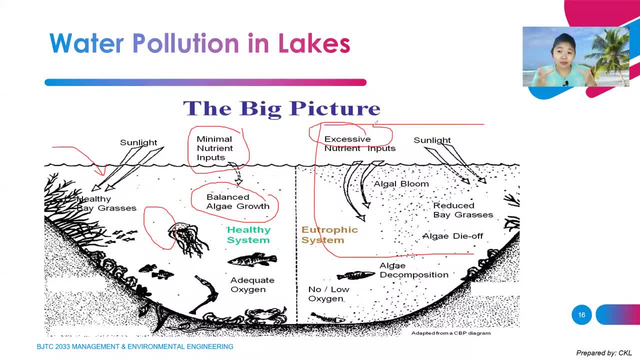 Can The Fish Still Survive? No, And Then Longer Times, When There, When It Dies, It Will Settle Downs, It Will Become Settle Downs. 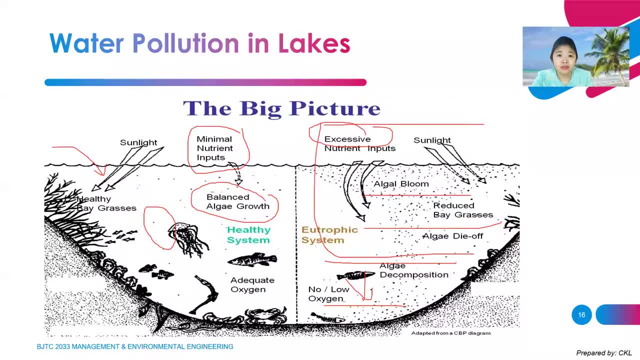 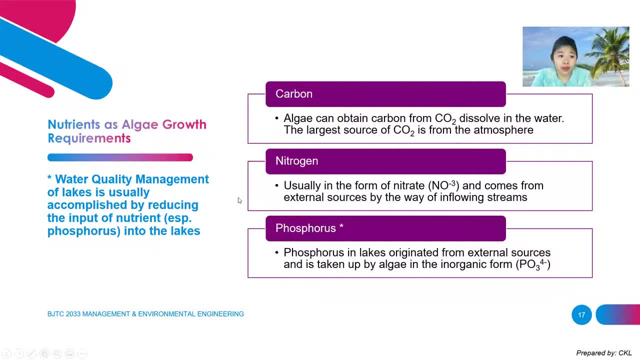 All These Things. So It Becomes. We Call It As The Neutrification. Okay, So Neutrin As A Nutrient Such As Phosphorus. So 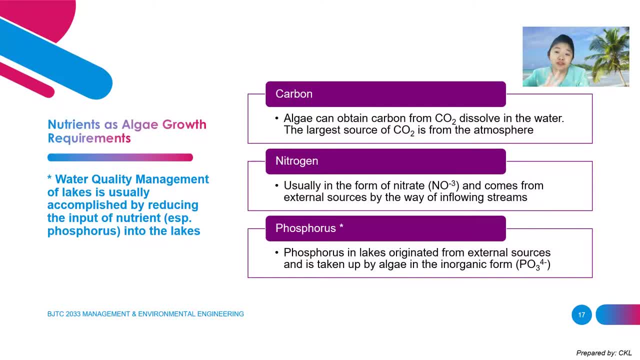 Very. The Phosphorus Come Is Actually Come From Our Fertilizer. So There Are Three Types Of Nutrients That Needed. So First Is Carbon. 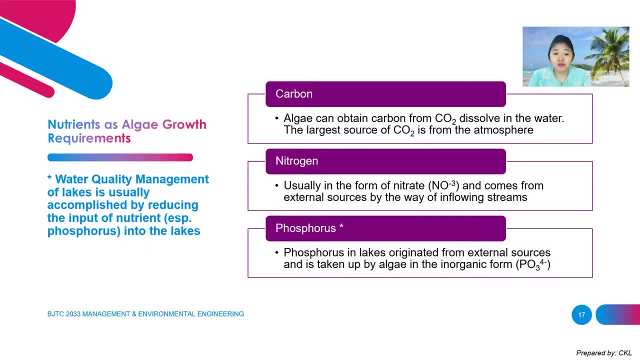 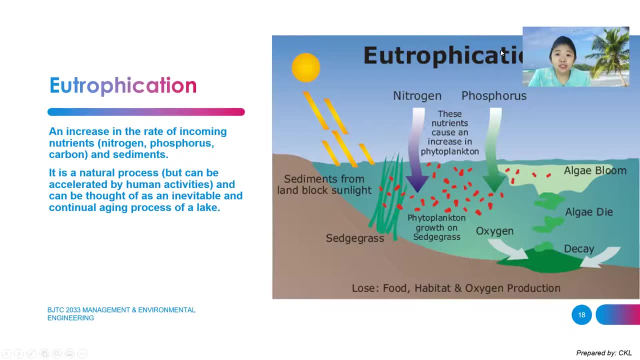 Second Of Inflowing The Stream. Phosphorus In The Lake Originated From The External Source Is Taken Up By The Algae In The Inorganic. 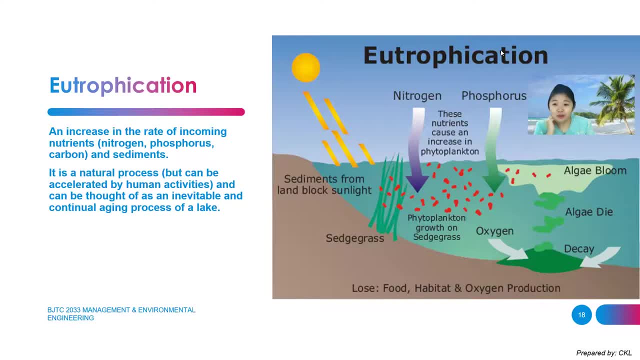 Form. Okay. So Neutrification Is Actually One Of This Full We Usually If Full Of Algae. So Because On The Surface You Will See. 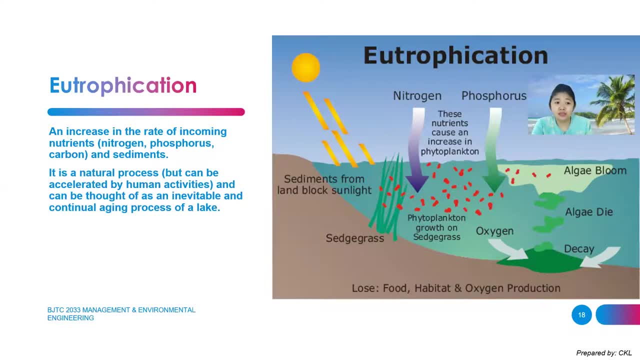 Like The Green Plants, More Plants, So That One Is Actually We Call Lake. A Lake Means Some Things That You Did. You Only Have Input. 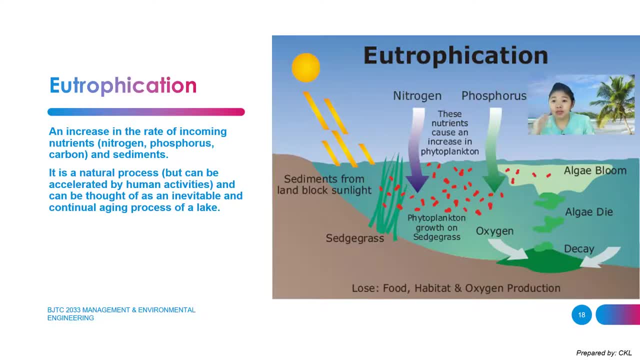 There Is No Output, So All The Waste Cannot Be Go Out. Once You Keep Putting Your Capacity Of The Lakes Will Become Smaller And 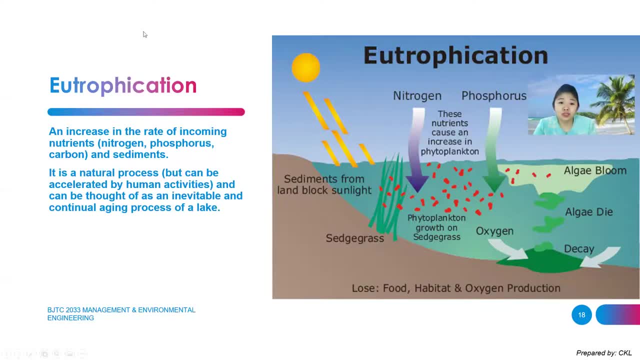 Smaller And Smaller, And Then Finally We Say As A Die: So That Is A Complete Process Of A Neutral Grass. So This Will Give. 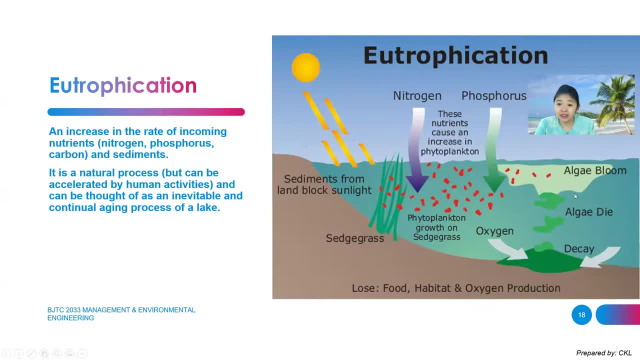 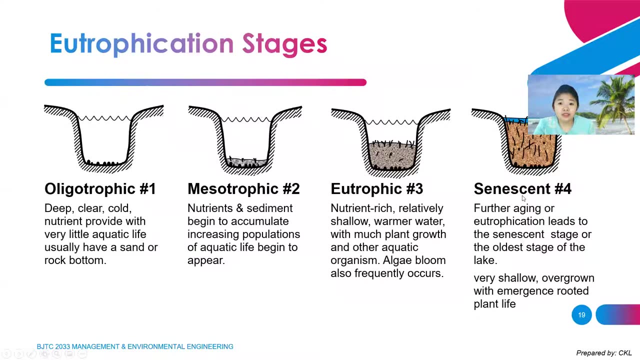 The Oxygen To The Algae, And Then The Algae Will Start To Bloom And Then It Will Die. So When It Dies, It Will Be. 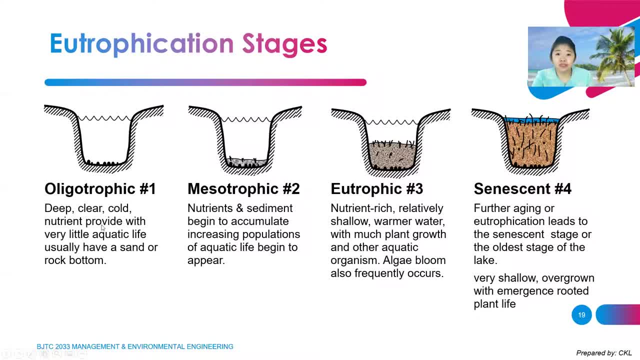 So You Have Very Deep And Clean And Cool And The Nutrients Provide With A Very Little Aquatic Life, So Usually You Still Can See. 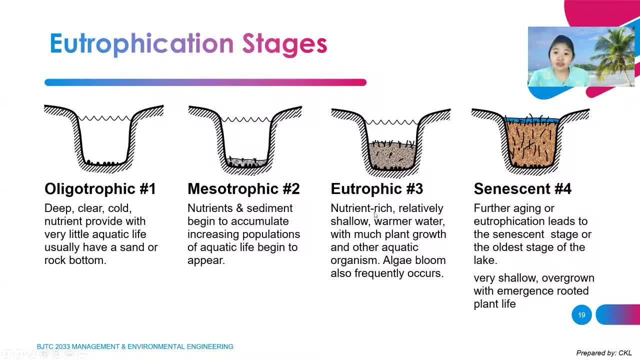 Through The Ascent And Become More. The Nutrients Become A Lot Of Nutrients So It Can Grow Very Fast. So The Relatives Become Swollen. 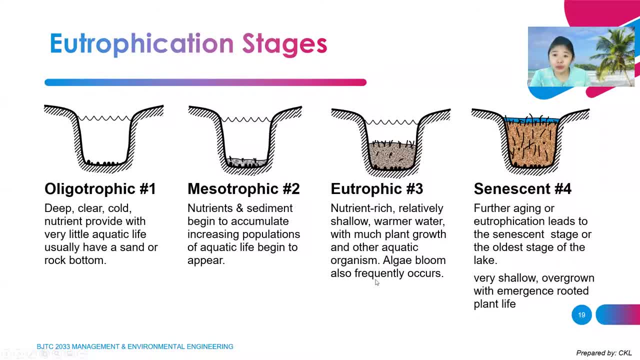 And Then, When You Have A Lot Of People, The Nutrification Leads To The Senescence Stage And The Oldest Stage Of The Lake. 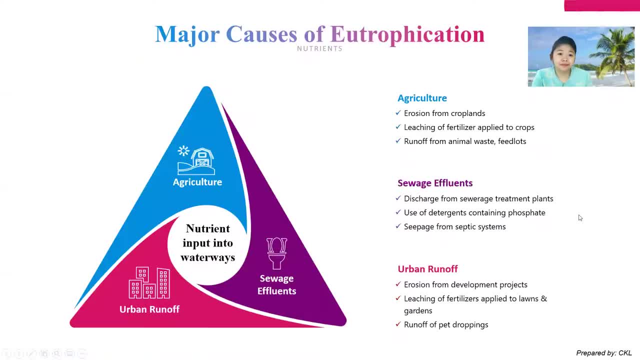 So It Become Very Swallow, Overgrown With Emergence Rooted Plant Life. So Usually When This Nutrients Coming From, So They Are Coming From. 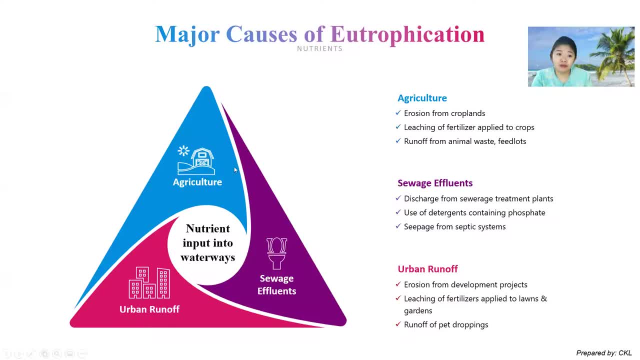 Three Places: First, Our Culture Activities. Second Is Our Sea, Which Affluence, And Then The One Is Our Open Run Off. So Run Off From 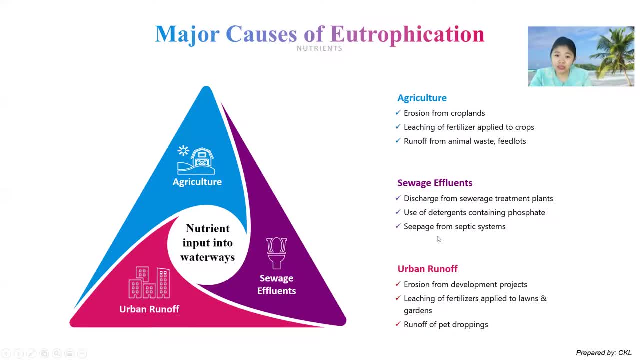 The Animal Waste Discharge From Sea Waste Treatment Plant Use Of Detergents: See Page From The System. So When You Go To Hotels You 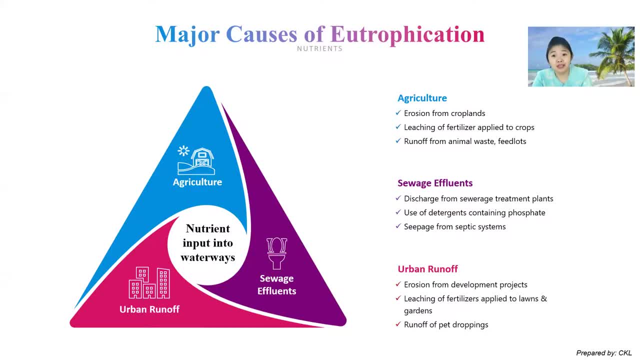 Might Be Thinking Less, So When They Wash Less, The Detergents That Been Used Will Be Less, So It Means That The Sewage Affluence. 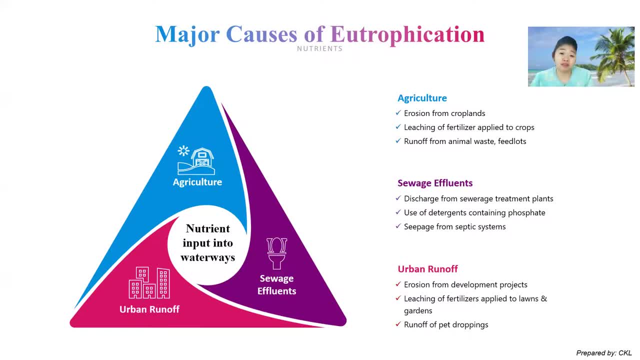 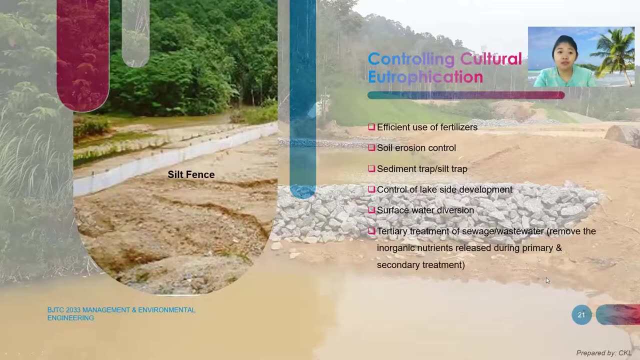 Will Be Reduced. Okay, So The Last One Is To That, If Not How It Grow. So This Is Something, And Then The Runoff From. 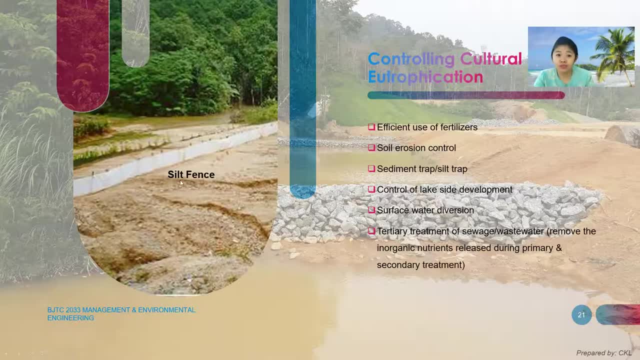 The Pet Droppings. Okay, So How We Control This Utrification. So First, So For The Usually At The Development Site You Will Have These: 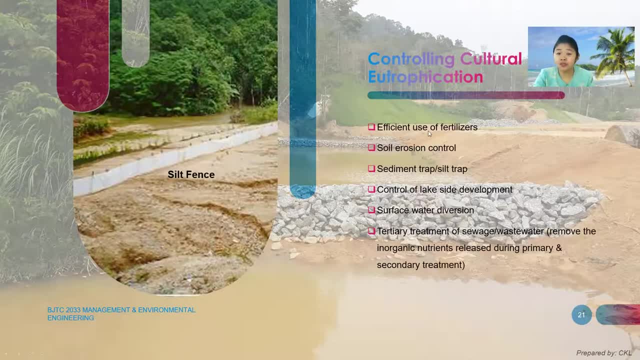 Seal Traps, So The Water's Coming Up, And Then You Will Start Here. Then Only We Release One Spline. Okay, So Now We Have. 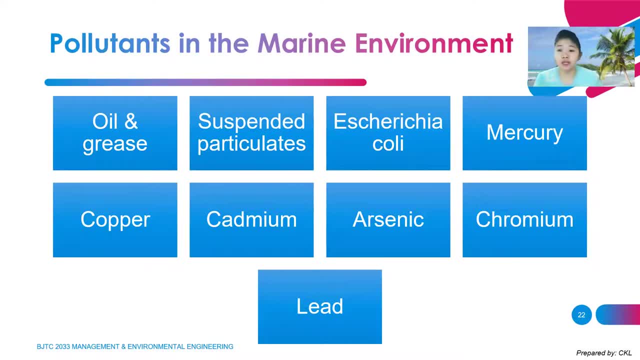 Our River, We Have Our Lake. Now We Going Into Sea, Our Marines, So The Sea We Get Our Seafood From Our Sea, Our Oceans. 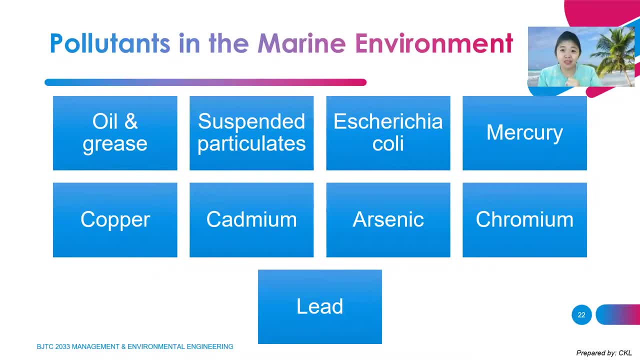 So We Reduce Our Plastic Waste, But Then We Set Plastic. There Are Still A Lot Of The Pollutants. Okay, Oil And Grease Suspended. 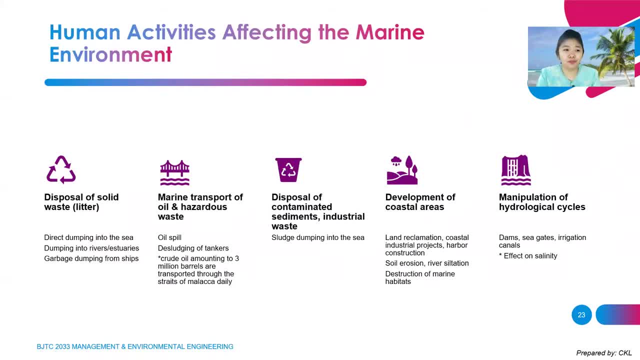 Particle Anterior Collie. No Disposal Of Solid Waste. Throw Everything Inside. Okay, So Direct Dumping Into The Sea, Dumping Into The River, All. 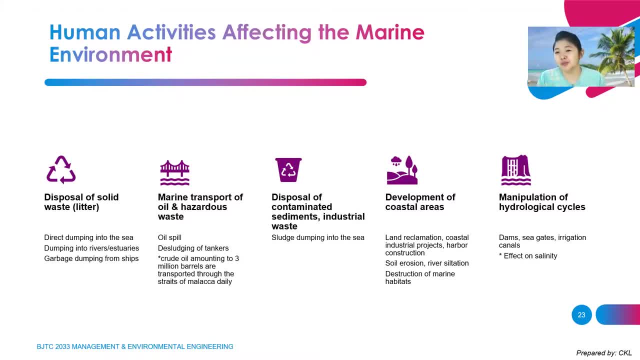 The Garbage Dumping From The Ship When You Go: Okay, So Second The Marines. Transport Of Oil And Hazardous Waste: Okay, So Oil Spill. 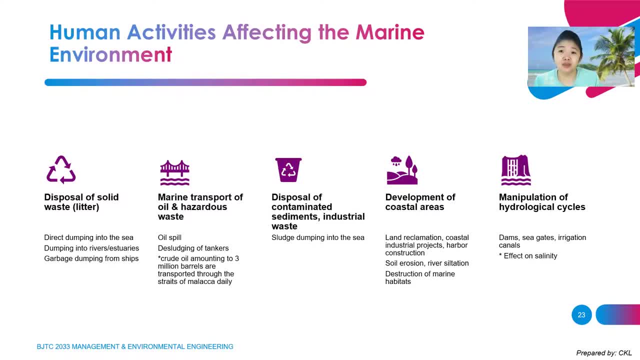 The Slush Of Tankles The Crude Oils Amounting Three Millions Barrel Are Transported. Actually, Accidents With The Ship, So The Leaking, So 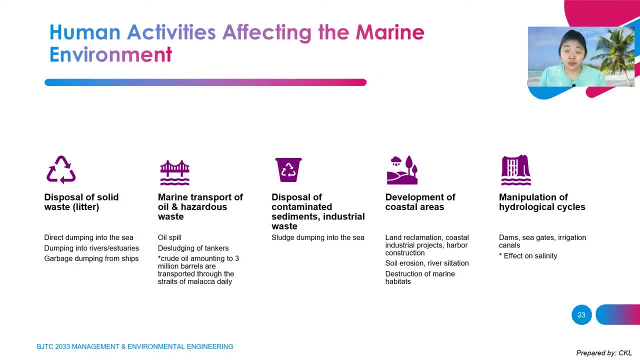 All Of This Is Actually Some Things Okay. So The Disposal Of The Contaminant Sediments Or Industrial Waste. So We Throw Everything To The 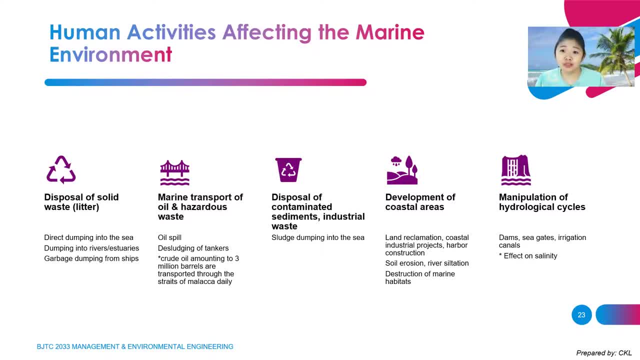 Sea. So It's Just Like Even Some Beach Are Getting Smaller And Smaller, Where The Sand Go Going Back To The Sea. Okay So 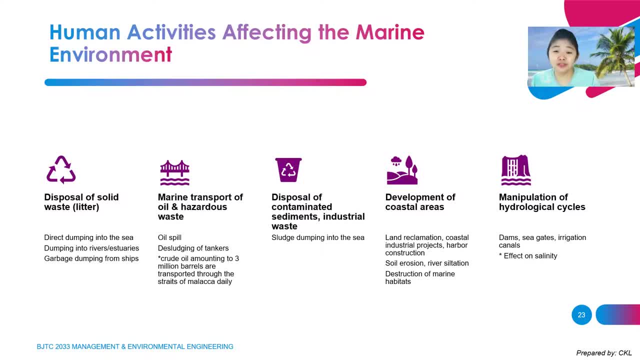 The Land Reclamation- One Of The Marine Pollution- Because You Have To Ball The Piling System That Using Is A Borrow Time, So When You 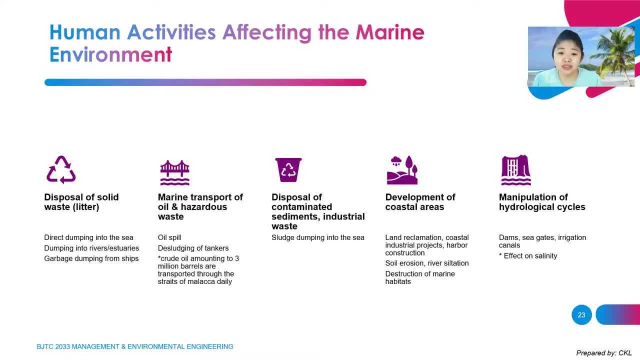 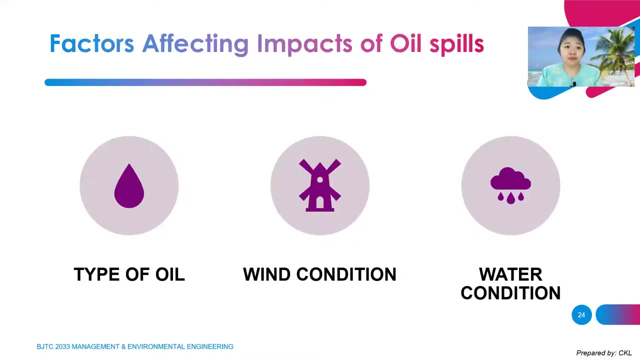 Borrow Where You Throw The, So You Borrow Time. So The Last One Is The Dam Seagate And Irrigation. Okay, Right, So The Factors That 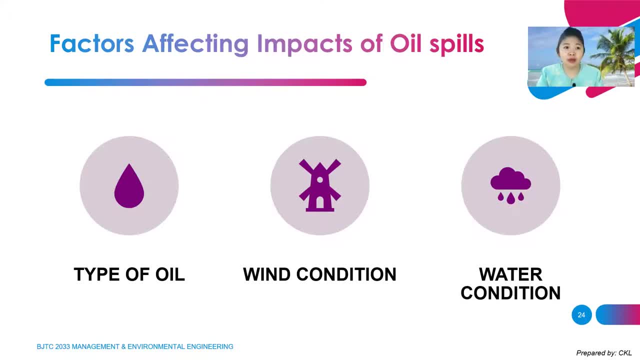 Affect The Impact Of The Oil Spill. So Oil Spill Is The Difference. Densities Will Provide A Difference Impact, Some Having A Very 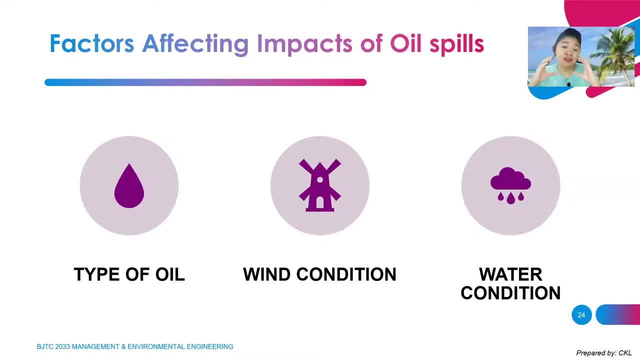 Thick One, So When You Having A Oil Spill On The Sea Can The Sunlight Go Through. It Will Be Helped To Spread Going. 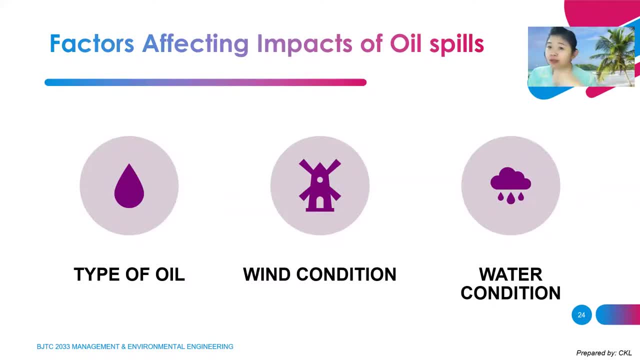 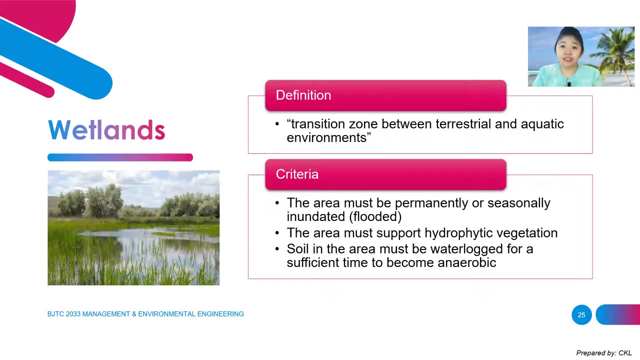 More Fast, Okay. Finally Is The Water Conditions. If The Water Is Cold, You Just Pour Some Oil In The Cold Water, And One Of The 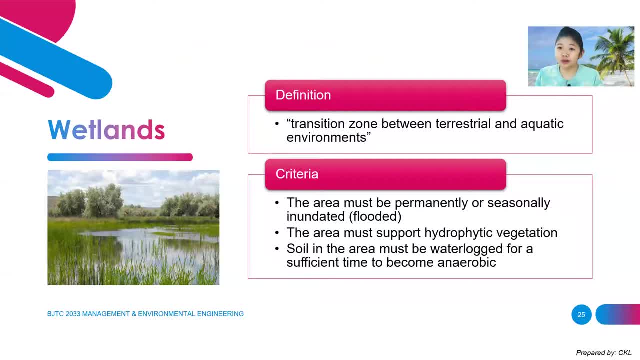 Methods Is Actually Been Implemented And Used As The For Us Not Only To Protect Our Seaside, But Then Also To Help Us To Recover. 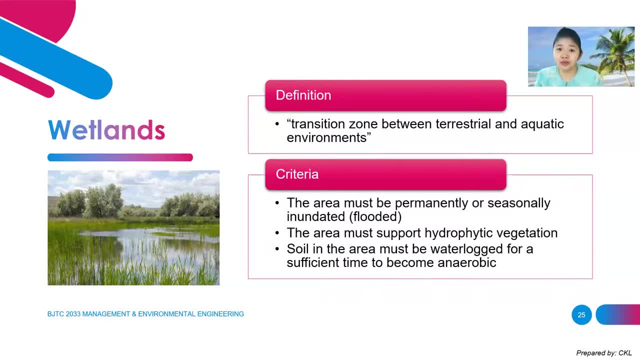 Our Wetland Is Actually A Transition Zone Between The Trust Terrestrial And Aquatic Environment, So Is Something That Between Us And Also Our Environments. 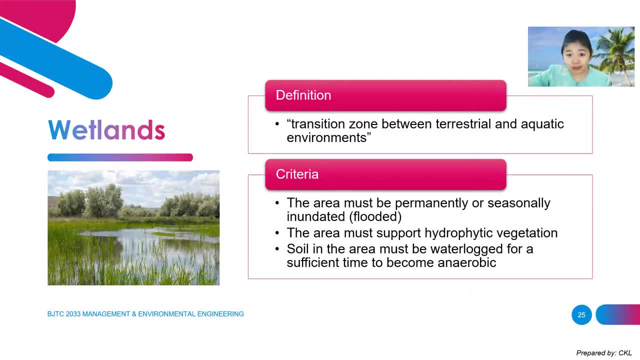 So The Criteria Is The Area Water Lock For A Sufficient Time To Become Anaerobic That You Can Capture The Water It Needs To. 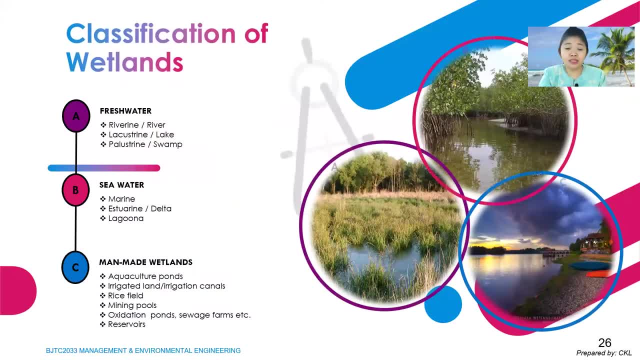 Be The Side That Can Capture The Water, Because We Need It, Is The Man Made Wetlands. Okay, So The Sea Waters, One We Have. 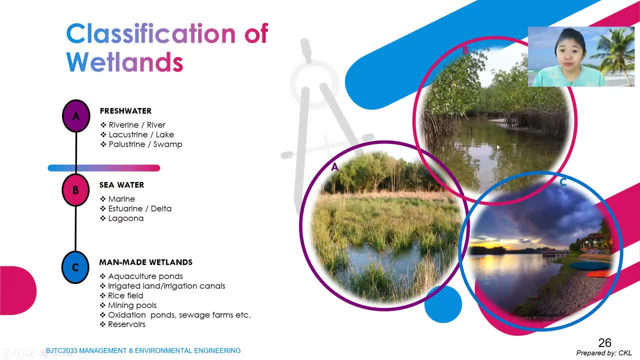 A River, We Can Use A River, So You Can See, Okay, First A. So See One, The Man Made One Is Actually We Have The. 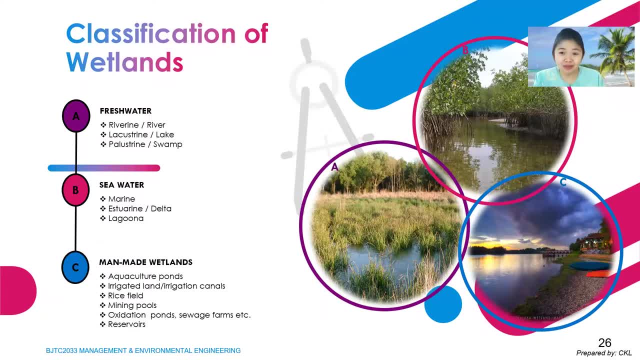 Most Biggest Wetland In Malaysia Is Actually Our Putrajaya. All Those Lake That You See In Putrajaya Is Actually Have In Malaysia And 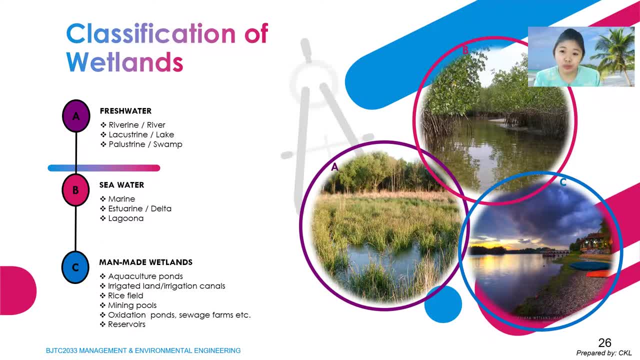 Then That One Is Actually A Man Made One. All Those Lake That You See Near To The Putrajaya Is Actually Not Originals Having 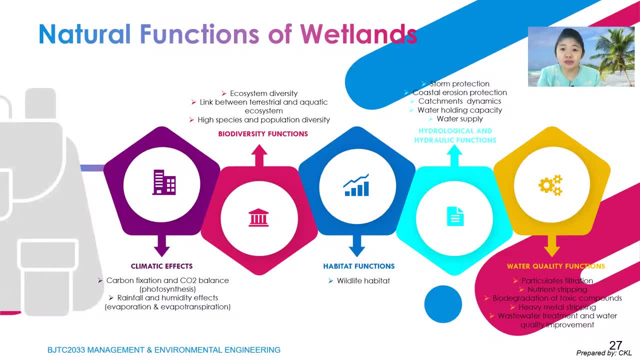 Water Wetland. Why We Need To Have Wetlands Is Actually, First, For The Climate Effects. It Will Help Us To Balance Our Carbon Dioxides. 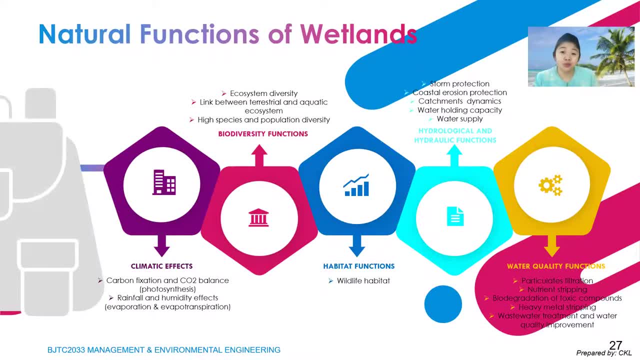 Because You Have A Lot Of Birds Or Others Ecologists To Come And Stay There. So The Ecosystem Diversity Link Between The Travicious And 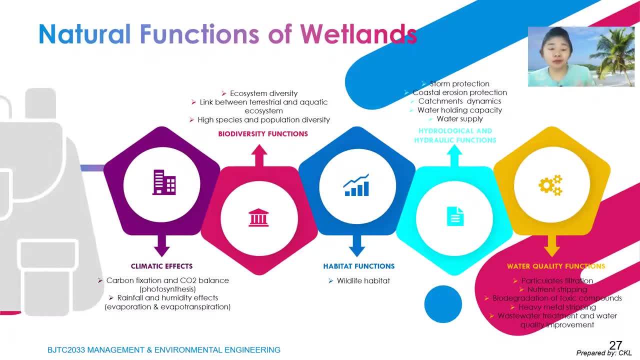 Aquatic Ecosystem And Then High Species And Populations Diversities. So Third One Is For Them: Some They Need Water, Some They Need Some. 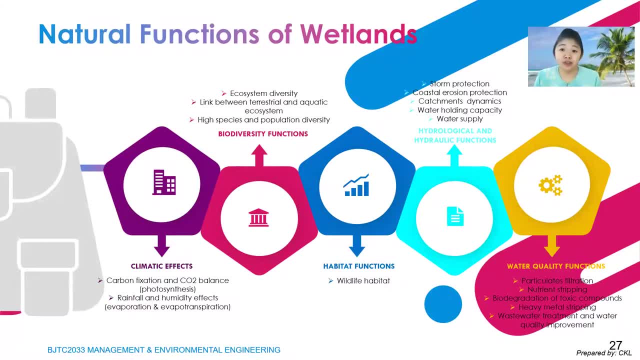 Trees, But Then When We Do Developments, We Actually Taking Everything From Them. So By Doing Wetlands, We Catchment Dynamic And Water Holding Capacity. 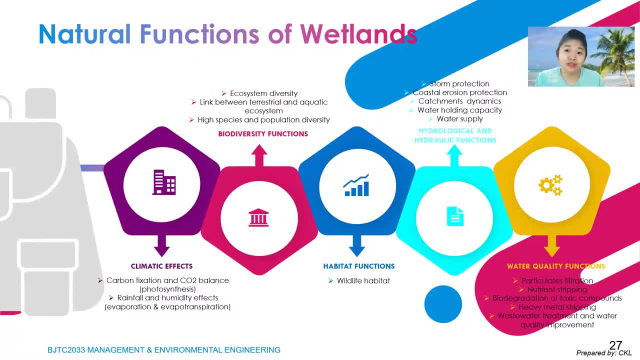 And Those That Successful, We Can Use At Water Supply. Example, The Putrajaya Water Is Actually Using Those From The Lake As The Food For 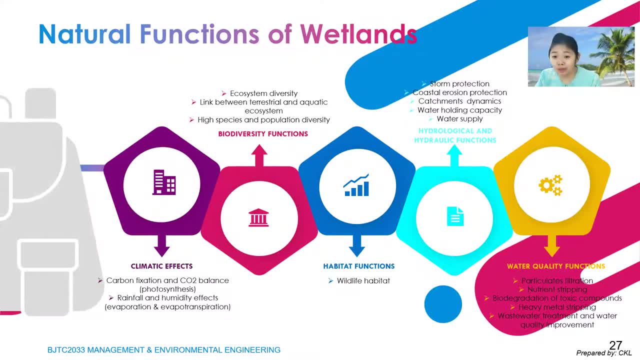 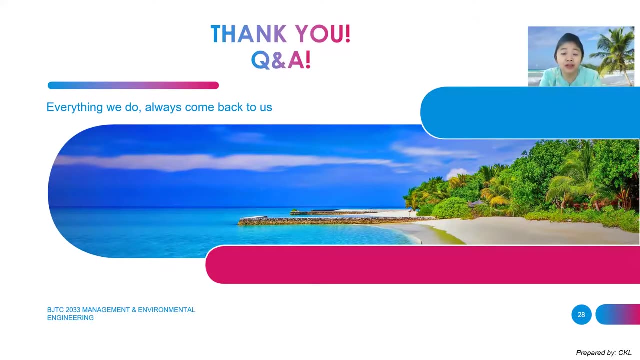 Them. So Okay, Biodegradations For The Toxic Compound, Heavy Matters Dripping And Waste, Water Treatment And Water Quality Can Be Improved, Right Okay. 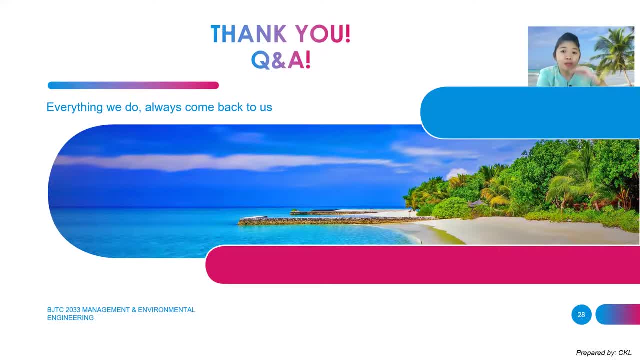 So That's All For Our Surface Water, Which Is River, And Then We Have Our Underground Water, Which Is Our. So The Waters That You 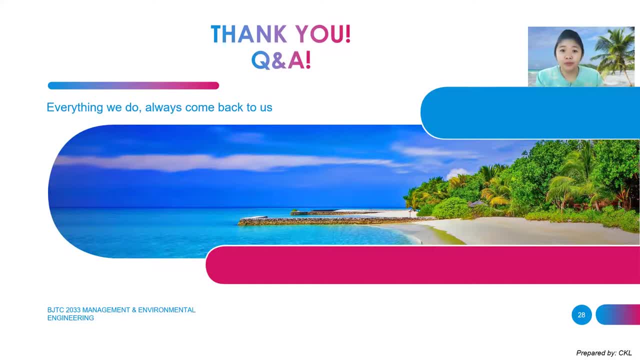 Cannot See That Located Underground, That Is Our Water And Water Can Be Improved And We Have All Water Which Is Our Water Can Be Improved. 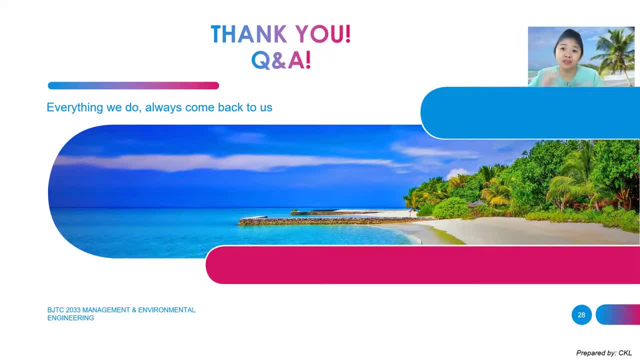 And We Have Water And Can Be Improved And We Have All Water Can Be Improved And We Have Water Can Be Improved And We Have. 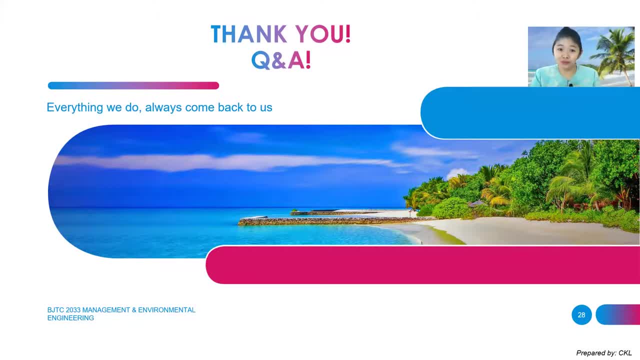 All Water Can Be Improved, And This Is Our Nay How Must Be Of. we can change the lake into a wetland system, into a successful system, a wetland system, the sustainable system. so at the same time, you also provide a new place, a new ecosystem to all the. 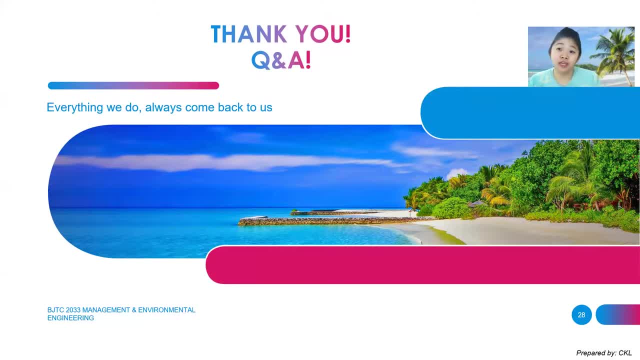 type biodiversity. so do you like this photo that I giving you now so you can see from the sea? so this, and then the last one is the sea pollutions. if you still would like to enjoy this kind of view, this kind of sea and beach, then I would only advise you guys, before you throw or before you do. 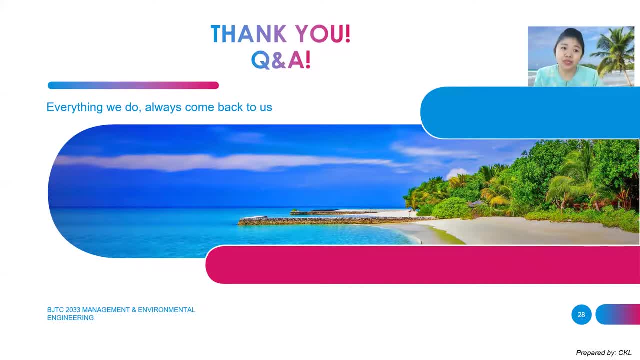 anything, please think, because everything that we do is always come back to us. so, if you will let you to, still would like to enjoy this nice view. then we have to think how we're going to protect our water resources, because water is some things that having the most related to our life. 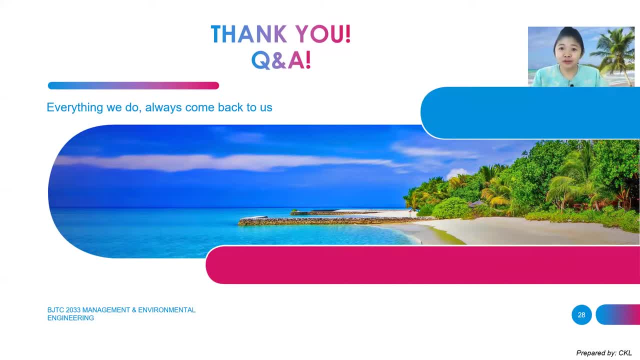 right, okay, so thank you for all of you. so if you have any questions, you can ask me through the whatsapp group or anything. all you can ask through the Google classroom. all right, I hope this is clear for you. you can actually compare on the slide that currently already have on in the online.